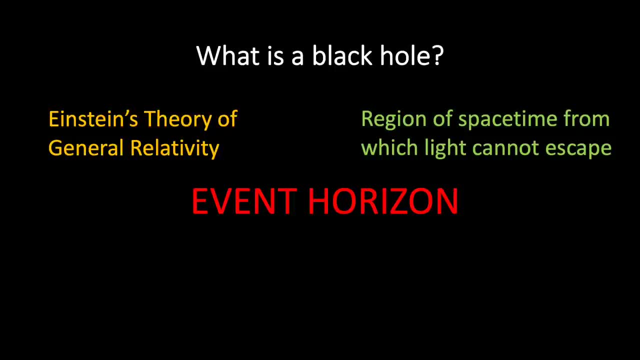 I was instantly hooked and desperately wanted to find out more. The only problem is that the physics of black holes, and in particular Hawking's work, is notoriously difficult and requires an advanced knowledge of Einstein's theory of general relativity as well as quantum field theory. But is it possible to determine the? 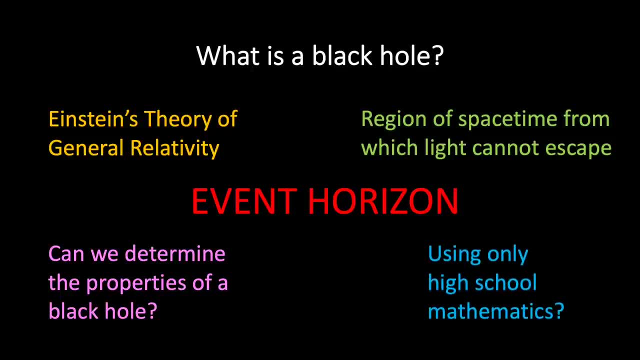 most exciting and mysterious properties of black holes using only advanced high school mathematics. Well, it turns out the answer is yes, and in this short video, I'd like to show you how. In fact, our strategy is quite simple. We are essentially going to guess the structure of the 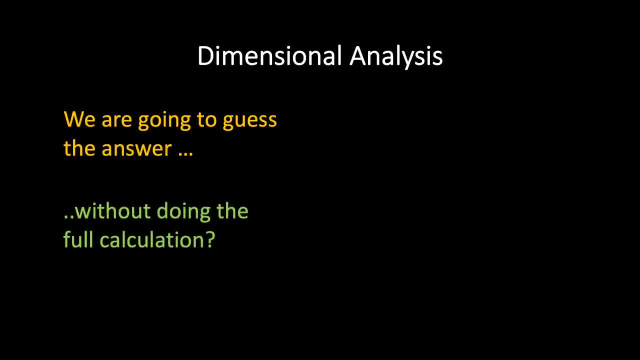 black hole equations without doing the full calculation, using a half-hour study of black holes. We are going to use a handy technique known as dimensional analysis. Dimensional analysis is perhaps the most valuable tool in a theoretical physicist's toolkit, as it allows you to construct equations without doing any of the hard work. 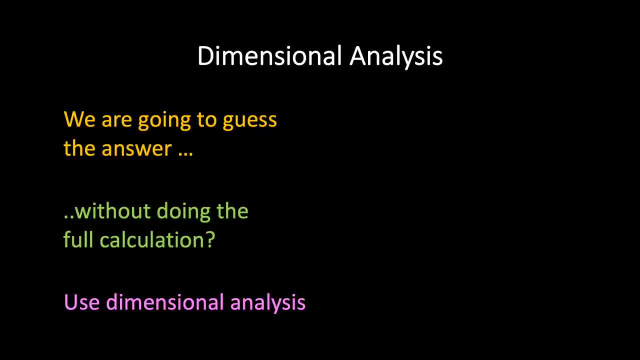 and, as you will see, it's remarkably successful. So how does it work? Well, the first thing to appreciate is that an equation in physics simply represents a relationship between physical properties, and a measurable physical property is referred to as a dimension. So what we're going to do is focus on the basic dimensions of length, time, mass and temperature. 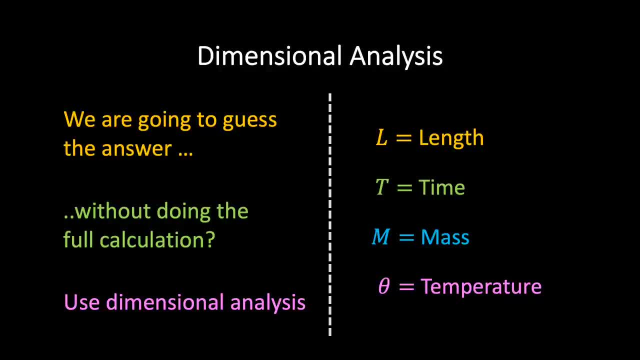 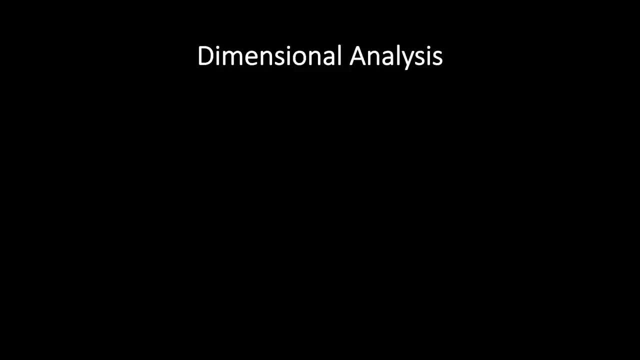 which we will signify with the letters L, T, M and theta. To understand what I mean by dimensional analysis, let's look at a simple example. The great thing about physics equations is that they provide a relationship between the dimensions of the properties appearing in the equation. 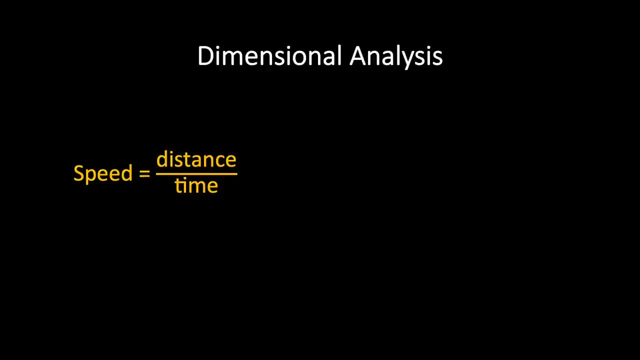 For example, consider the equation: speed equals distance divided by time. To determine the dimensions of speed, we refer to the defining equation, which tells us that the dimension of speed is equal to the dimension of length divided by time. Square brackets are used to signify that we are interested. 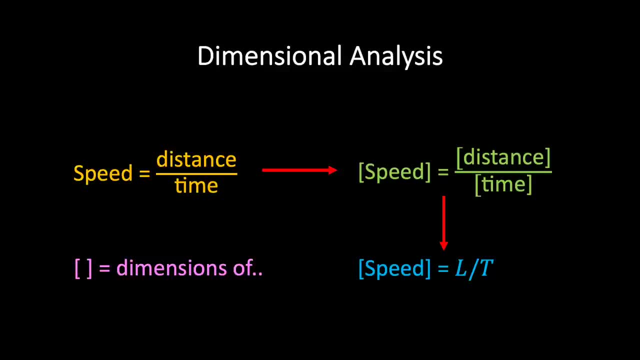 in the dimension of the quantity inside the bracket. Now it turns out that some physics equations are special in the sense that they contain what are known as fundamental constants. A fundamental constant is a physical quantity that is believed to be universal in nature and constant in time. 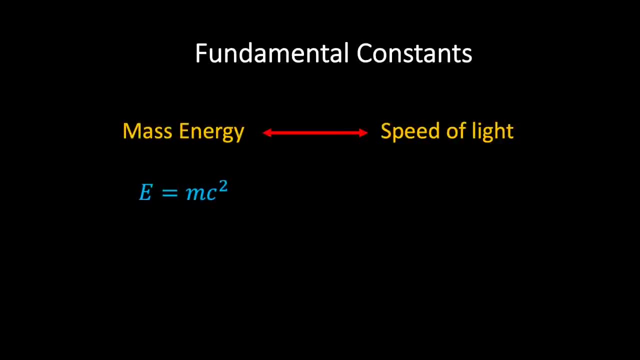 The most famous example being the speed of light, which appears in the famous equation, equals mc squared. This equation allows us to calculate the mass energy of an object if we know its mass. The speed of light c is a fundamental constant that tells us the 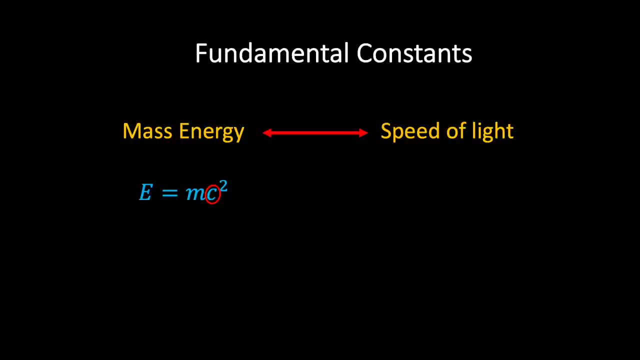 exchange rate between mass and energy. Since c refers to a speed, the dimensions of c can be written as c equals L over T. We also note that we can use the equation equals mc squared to determine the dimensions of energy, which can be written as m L squared over T squared. 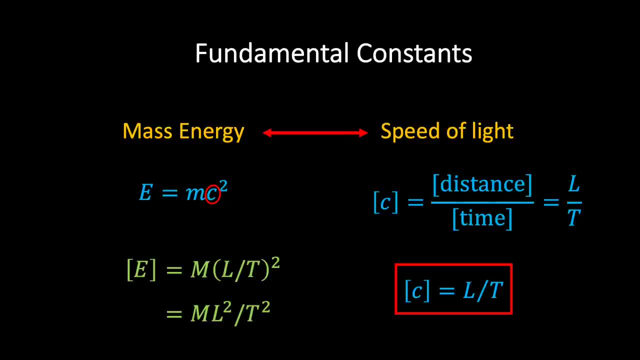 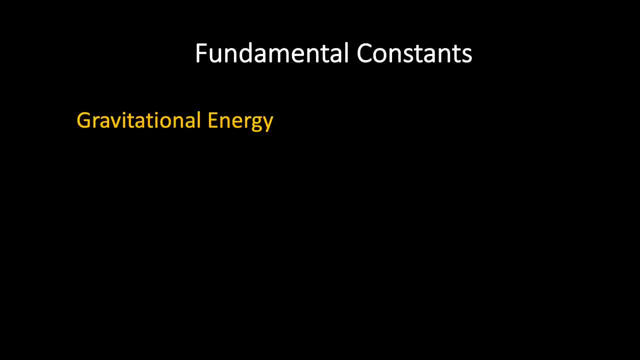 Let's now use this dimensional information to explore some of the other fundamental constants that will prove crucial to our understanding of black holes. Firstly, consider the gravitational potential energy that exists due to the relative position of two or more masses If two masses are separated by a distance r. 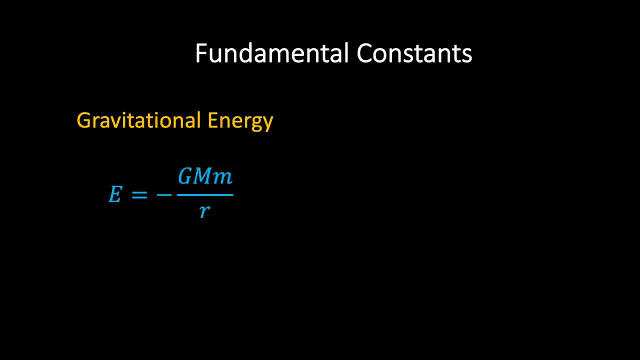 then the gravitational potential energy can be calculated using the equation: e equals minus g, M m over r, where g is Newton's gravitational constant. By rearranging this equation and inserting the dimensions of energy that we calculated previously, we find that the units of g are equal to L cubed over m t squared. 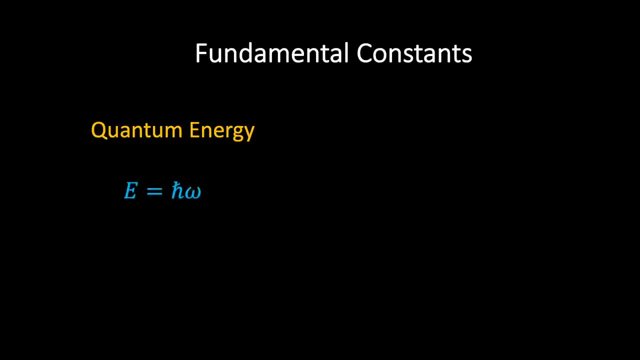 Next, consider the famous quantum energy relation. E equals h bar omega, which relates the energy of a quantum of light to the frequency of the light. Here, h bar is the reduced Planck's constant. In order to determine the dimensions of h bar, we simply rearrange the energy equation. 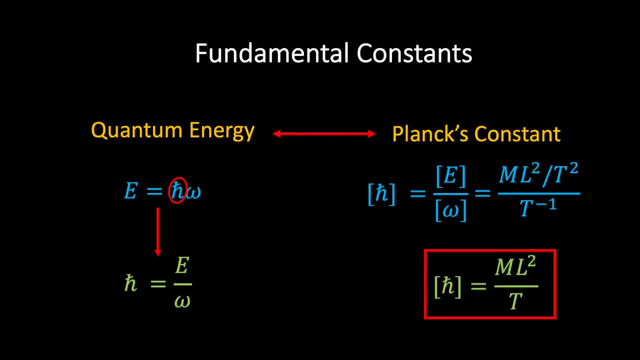 and since frequency has dimensions of inverse time, we see that the dimensions of h bar is m L squared over t. The final fundamental constant that we will be concerned with relates to the field of thermodynamics and, more specifically, systems of large numbers of particles, According to, 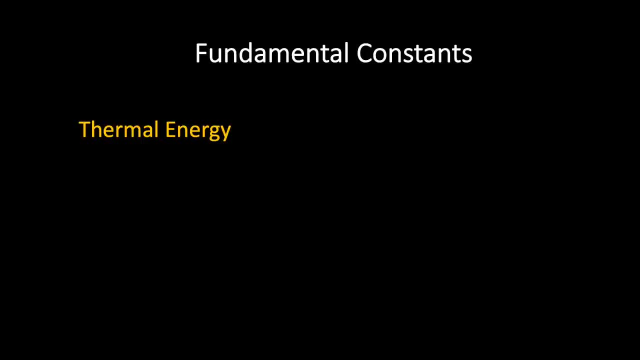 the kinetic theory of gases. for a system of n particles at temperature t, such as a gas, the thermal energy is related to the temperature by the equation: E equals three over two: n, k, t, where k is Boltzmann's constant. By rearranging this equation for Boltzmann's 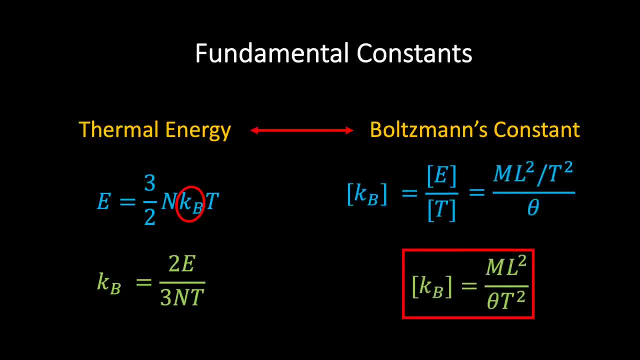 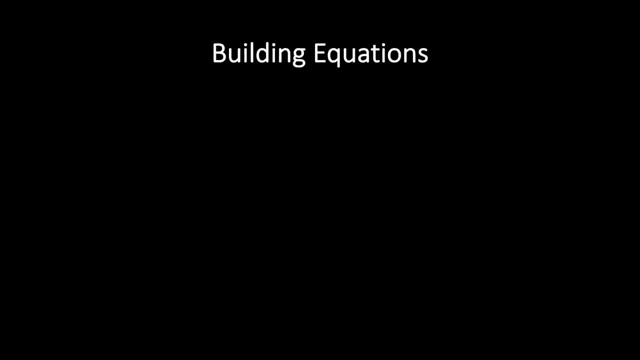 constant. we see that the dimensions of Boltzmann's constant is given by m L squared over theta t squared. Having laid the necessary foundations, we're now in a position to start building equations using the fundamental constants as our building blocks. The rules of the game are as follows: When using dimensional analysis to construct equations, 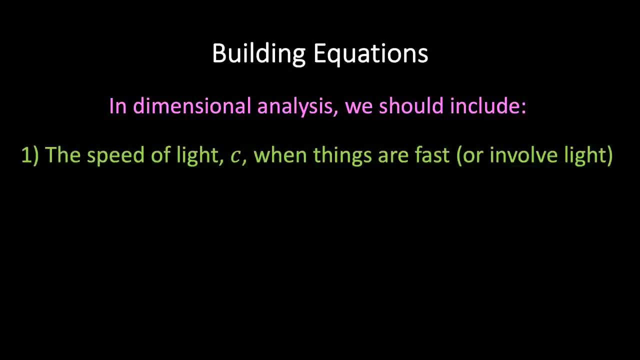 we should include the speed of light c when things are moving fast or involve light. We should include the gravitational constant g when things are massive. We should include Planck's constant when dealing with quantum systems and we should include Boltzmann's. 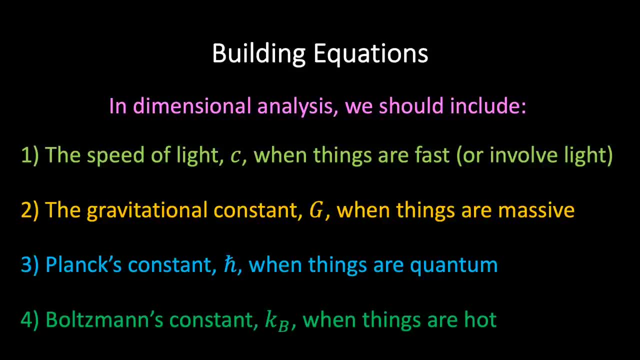 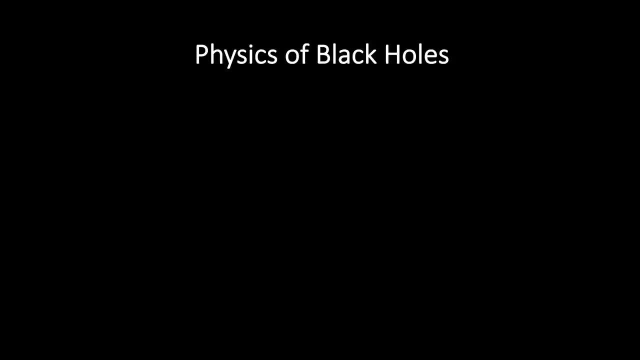 constant when things are hot. It sounds simple, so let's get started. Our objective is to uncover the properties of black holes using dimensional analysis. The good news is that the properties of black holes are very similar to the properties of black holes using dimensional analysis. The problem is that our task is made significantly. 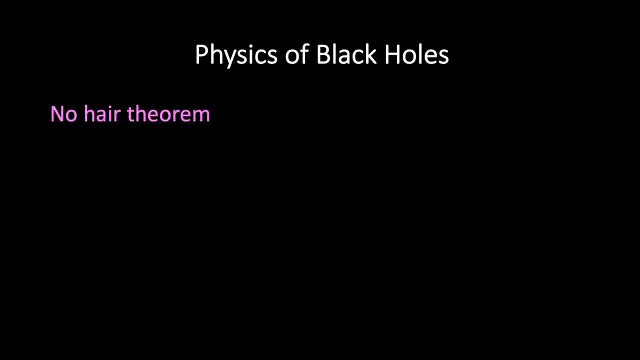 easier because of a famous theorem known as the No-Hair theorem. The No-Hair theorem states that all black hole solutions in general relativity can be completely characterized by only three externally observable classical parameters: mass, electric charge and angular momentum. All other information, for which hair is a metaphor about the matter that 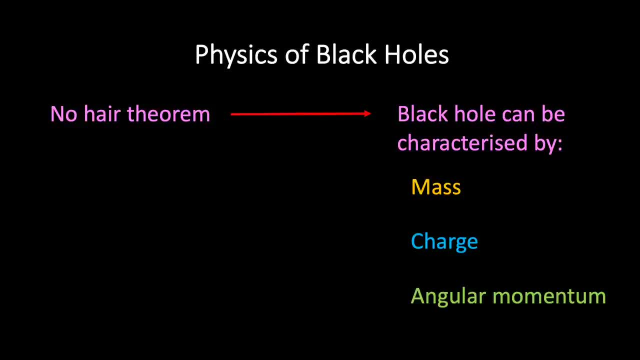 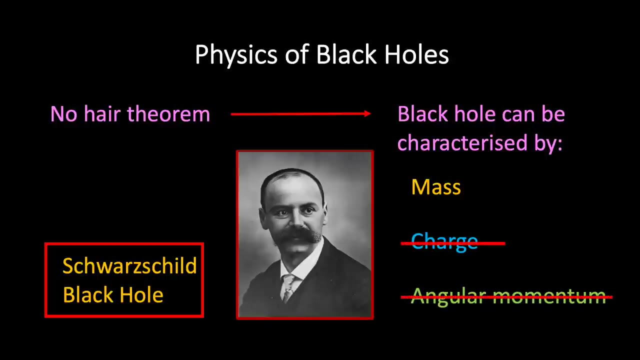 formed, the black hole disappears behind the black hole event horizon and is therefore permanently inaccessible to external observers. In what follows, we will focus on a special class of black holes, known as Schwarzschild black holes, which have neither electric charge nor angular momentum, and therefore a Schwarzschild black hole is completely characterized by 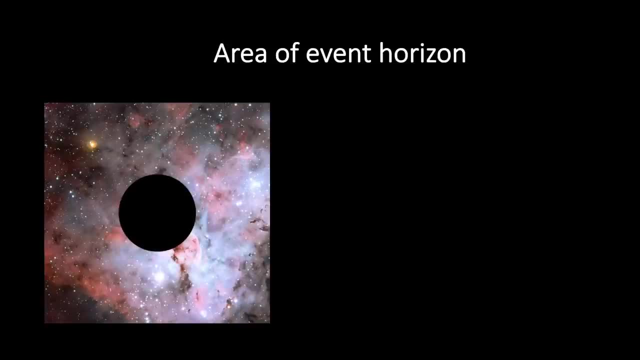 its mass. Armed with the No-Hair theorem and dimensional analysis, we are now in a position to answer the following question: What is the area of the event horizon of a black hole? Well, firstly, black holes are clearly massive objects, and so our equation should include: 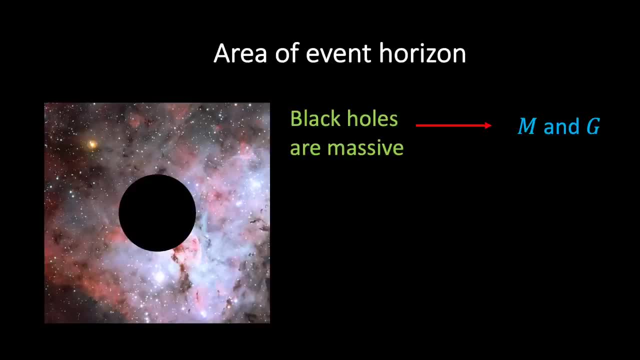 Newton's gravitational constant g, along with the characteristic mass of the black hole, m. Furthermore, we know that a black hole is a region of spacetime where gravity is so strong that nothing, not even light, can escape, and so we should expect the speed. 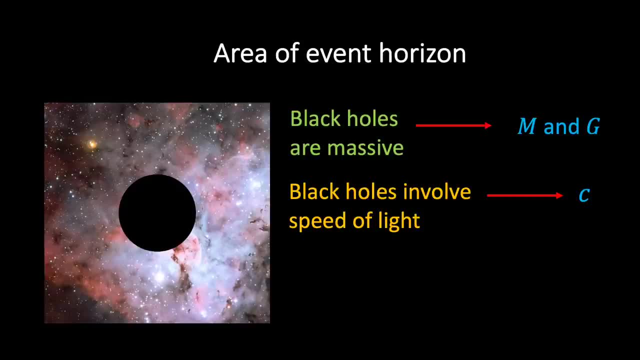 of light to feature in our equation. Our strategy is to write the area of the event horizon as a equals g to the power alpha, times c to the power beta, times m to the power gamma, and then we will use dimensional analysis to determine alpha, beta and gamma. So let's do that. To fix alpha, beta and gamma, we simply need: 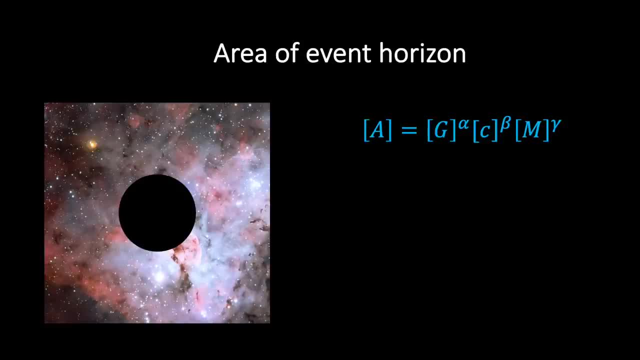 to match the dimensions on either side of this expression. The left hand side represents an area which has dimensions of length squared. For the right hand side, we need to insert the dimensions of g and c that we calculated earlier. If we do that, then we find the following green expression: 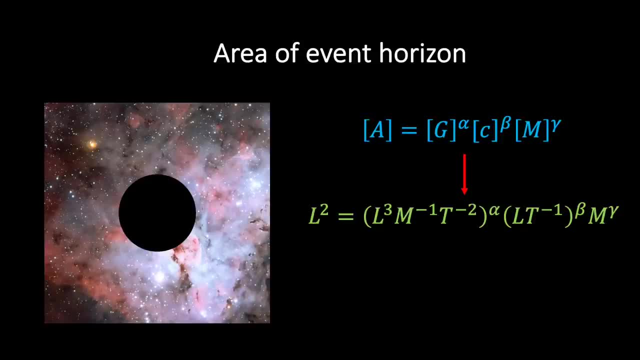 We can then use the law of exponents to gather terms and simplify this expression, in which case we find the following: Now, since the dimensions on both sides of the equation need to match, this places a set of constraints on alpha, beta and gamma. To make this clear, we can imagine writing: 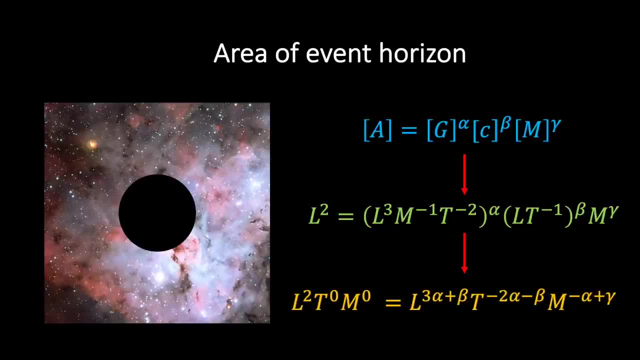 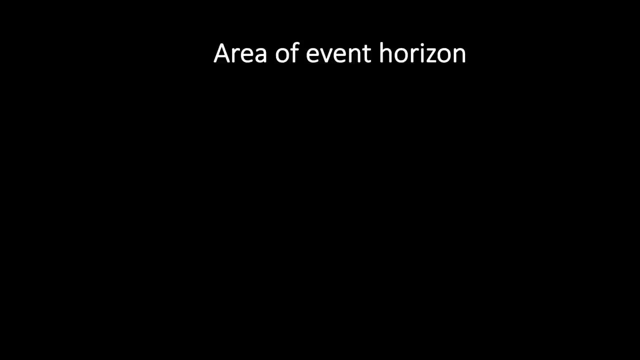 the left hand side in an equivalent form as follows: We can do this because any quantity raised to the power of zero is simply equal to one. If we then match up the exponents of l, t and m, we find a set of three simultaneous equations which can be solved by substitution After a. 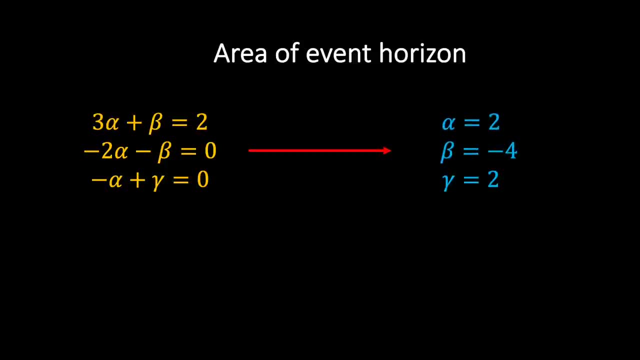 little bit of algebra, we find that alpha equals two, beta equals minus four and gamma equals two. If we then sub these values into our original expression, we find that the area of the event horizon of a black hole is proportional to g squared m squared divided by c, to the power of 4.. 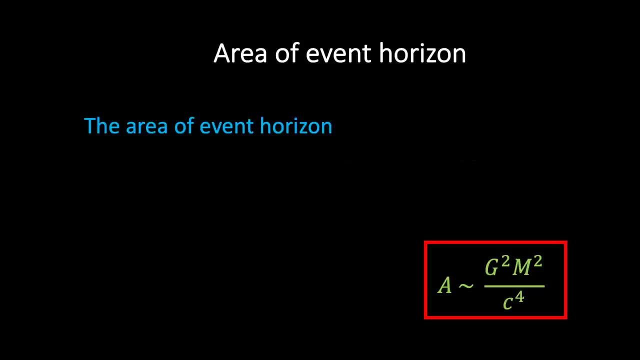 In other words, the area of the event horizon will increase as more mass falls into the black hole. More specifically, we see that if the mass of our black hole doubles, then the area of the event horizon will quadruple, and so we begin to see the power of dimensional analysis, Although we don't. 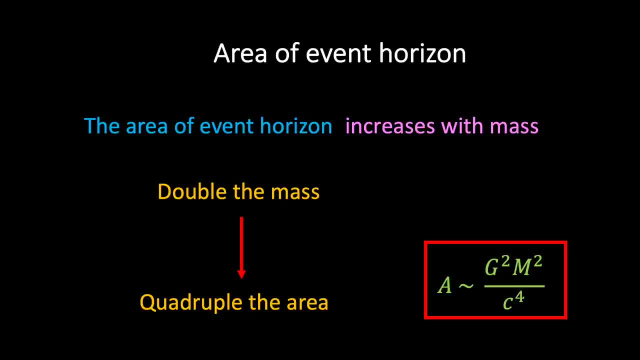 know the exact value of the proportionality constant appearing in the mass area expression. dimensional analysis does allow us to determine the structure of the relationship, and often this is the most important part of an equation. It's interesting to note that a detailed calculation of the black hole event horizon will be the most important part of an equation. It's interesting to note that a detailed calculation of the black hole event. 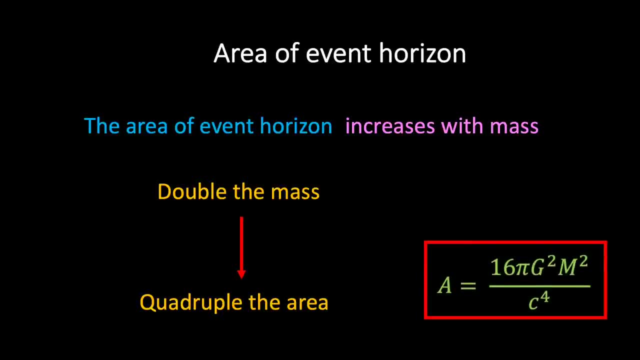 horizon yields the following exact expression: and we see that the structure of this expression does indeed match the one derived using dimensional analysis. So why is this mass area relationship important and what is it telling us about black holes? Well, the first thing to appreciate is that 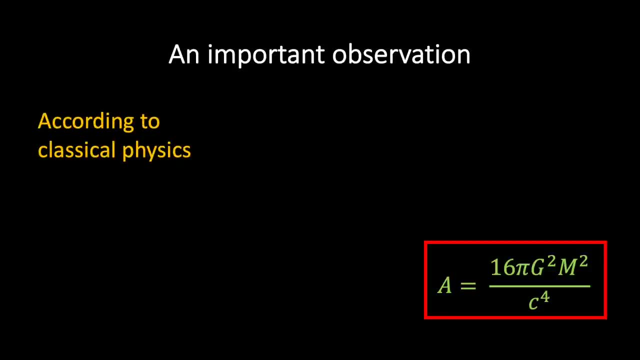 from a classical point of view, nothing can ever escape from inside the event horizon of a black hole and therefore in all physical processes, the area of the event horizon can only ever increase. It can never decrease. Now, the idea that there exists a quantity that can only ever increase with time. 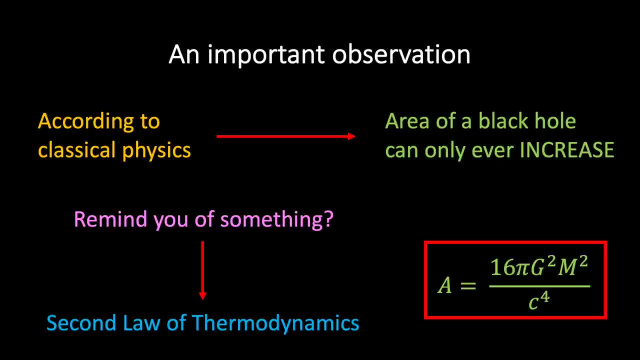 might remind you of the second law of thermodynamics, which states that the entropy of an isolated system must increase with time. Because entropy is such an important concept and a key part of our analysis of black holes, it's worth taking a short detour to understand the concept in a bit. 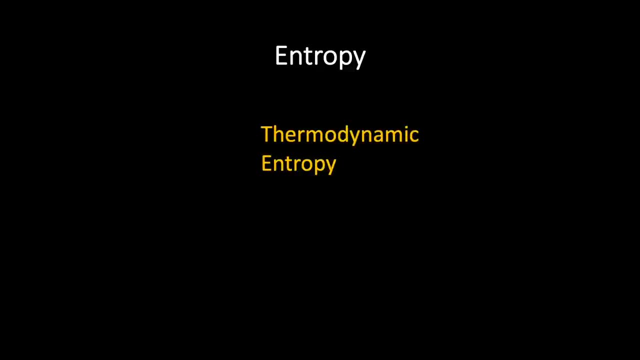 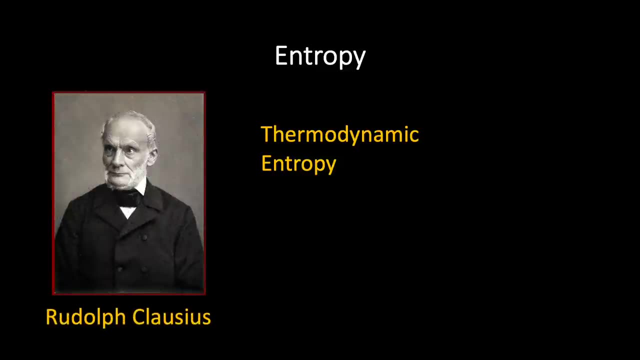 more detail. The concept of thermodynamic entropy was first introduced into gas dynamics by the German physicist Friedrich Nietzsche. The concept of thermodynamic entropy was first introduced into gas dynamics by the German physicist Friedrich Nietzsche. Rudolf Clausius Clausius had introduced the concept to describe the flow of heat. He originally 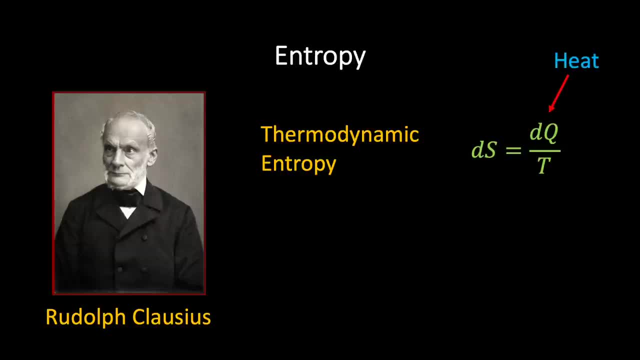 defined the change in entropy of a system as the heat energy it absorbed divided by the temperature at which it absorbed the heat. The remarkable discovery of Clausius was that, because heat always moves from high temperature regions to low temperature regions, the total change in entropy summed over all the parts of the system that were exchanging heat with one another was always positive. 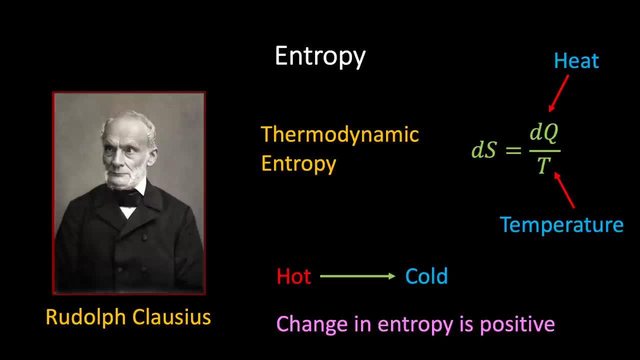 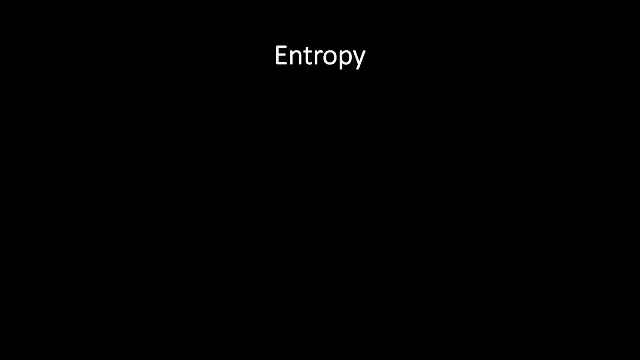 summed over all the parts of the system that were exchanging heat with one another was always positive. The entropy was always increasing. But why is this true? Although Clausius had successfully introduced the mathematical definition of entropy, he was unable to provide a fundamental explanation of why the second law of thermodynamics was true. 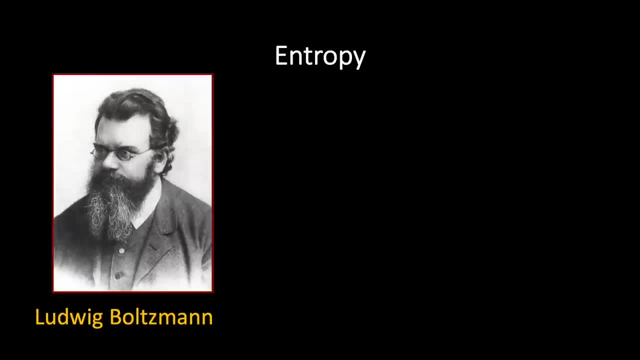 However, in 1877, the Austrian physicist Ludwig Boltzmann provided a beautiful explanation of entropy in terms of the microscopic components of a physical system. According to Boltzmann, the entropy of a system is simply characterized by the number of ways of rearranging the microscopic components of the system in such a way that some macroscopic feature. 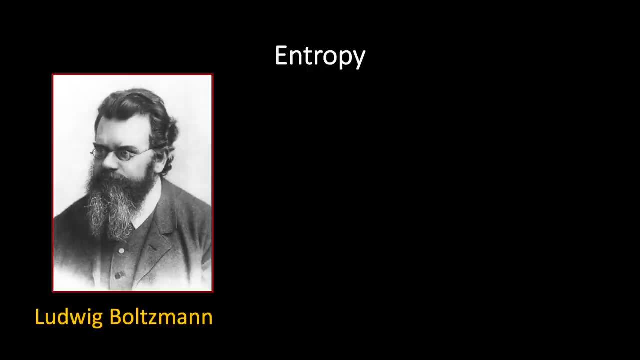 such as the pressure or temperature, remains unchanged. This statement is encoded in Boltzmann's famous entropy law, which can be found etched into his gravestone. According to Boltzmann's definition, the entropy of a system is equal to Boltzmann's constant multiplied by the logarithm of w. 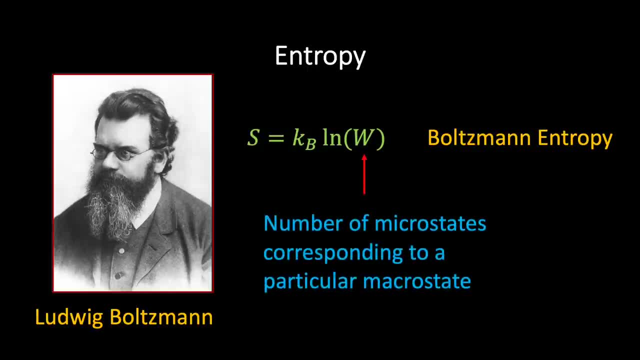 w is the number of microstates corresponding to a particular macrostate. To make this a bit clearer, imagine the bottom of a box is completely covered with red and green marbles. Now imagine that you arrange the marbles so that the left half is green and the right half. 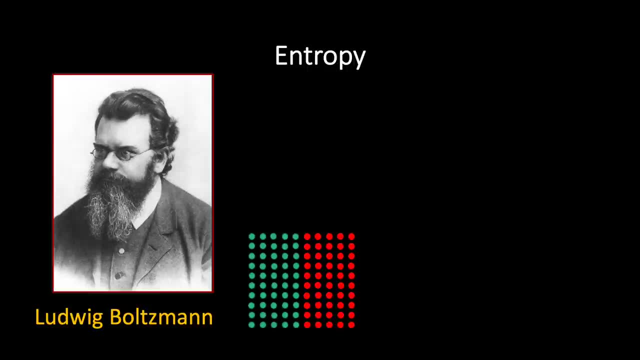 is red. This corresponds to a particular appearance or macrostate of the system. Let's label this macrostate as the split-state. If we then shook the box of marbles so that the two sets of marbles became one, came thoroughly mixed together, we would see a random arrangement of the marbles which we might. 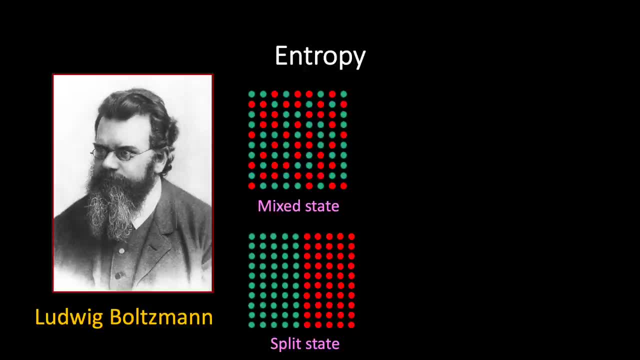 label as a mixed macrostate. If we then shook the box again, we would get a different arrangement of the marbles, but we would still label the macrostate of the system as being mixed. In fact, there are a huge number of marble configurations or microstates corresponding to a mixed macrostate. On the other, 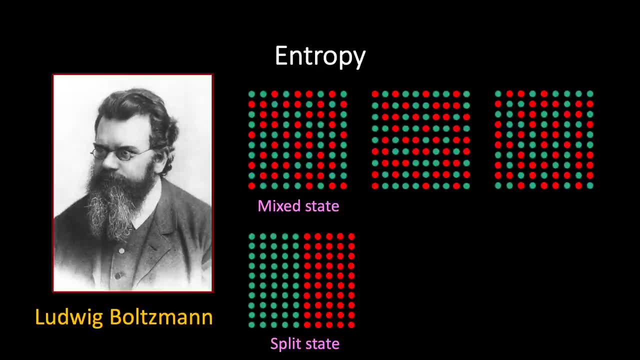 hand, there are clearly fewer ways for the marbles to arrange themselves into the neatly separated split state. Boltzmann's great insight was to realize that he could define the entropy as the number of microstates corresponding to a particular macrostate: Fewer microstates. 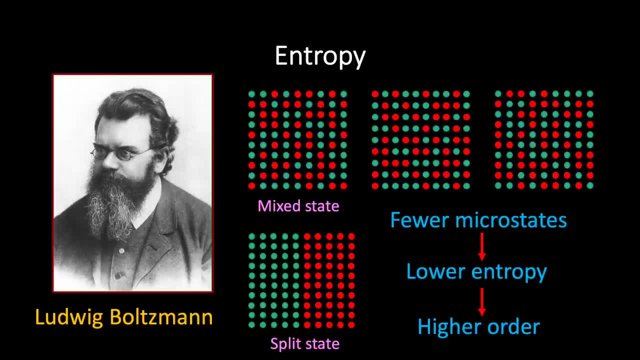 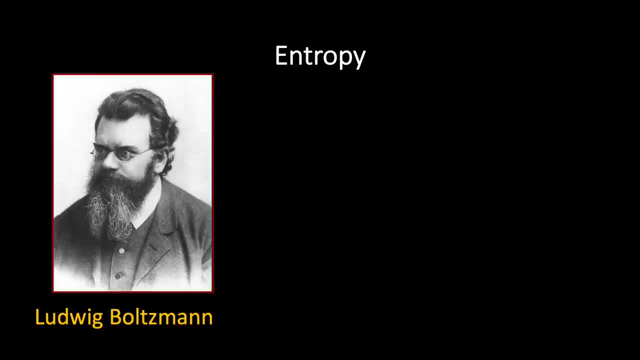 corresponds to lower entropy and therefore more order in the system. So what has this got to do with black holes? Well, you can think of a black hole as a universal wastebasket that swallows up information as matter falls inside, Since a black hole refuses to tell us what has fallen inside. 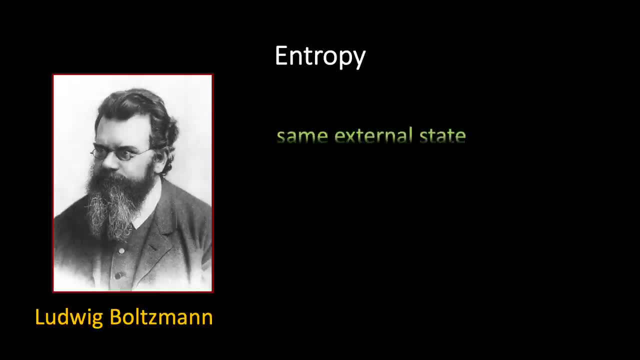 we can view a black hole as a system that has the same external state for lots of possible internal states. This suggests that the black hole may have a very large entropy value. But exactly how large? Well, we've already uncovered the first clue when we discover that the area of the horizon 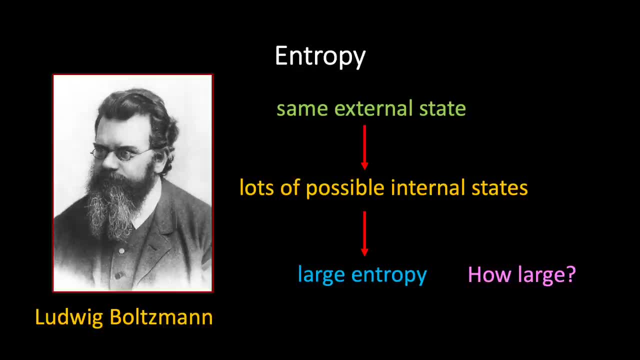 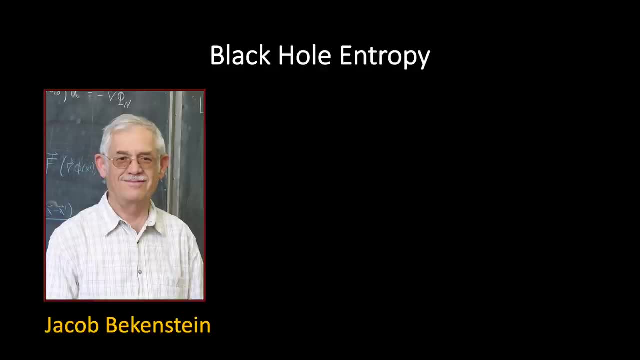 of the black hole always increases when mass falls inside. In 1972, Jacob Bekenstein, an Israeli physicist, proposed that it does indeed make sense to have a black hole as a system that has the same amount of energy as a black hole. So what does that mean? Well, the first thing we need to do is 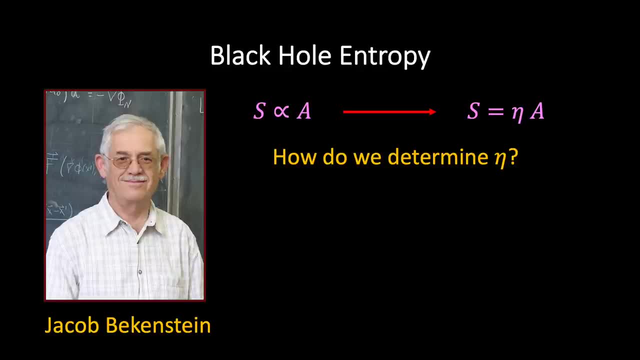 determine the dimensions of entropy, since this will then allow us to figure out the dimensions of eta. To do this, we refer back to the thermodynamic dimension of the black hole, So we can look at the thermodynamic definition of entropy. ds equals dq over t, which tells us that entropy. 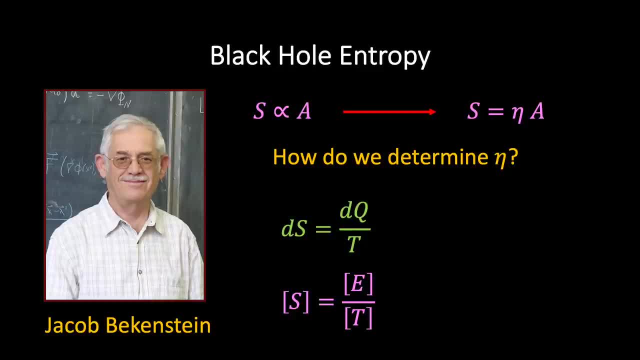 has dimensions of energy divided by temperature, And so we find that the entropy has dimensions of ml squared t to the minus 2, theta to the minus 1.. We can then use this to determine the dimensions of eta, since eta is equal to the entropy divided by the area, And so we 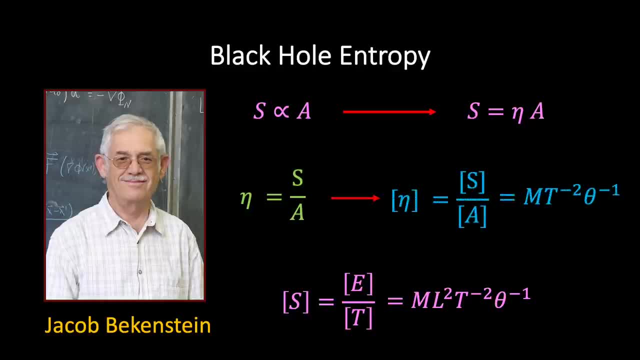 see that the dimensions of eta must be mt to the minus 2, theta to the minus 1.. Furthermore, we know that eta is constant. therefore, eta must be constructed from quantities which are themselves constant in time. This provides a strong hint that eta can be built using 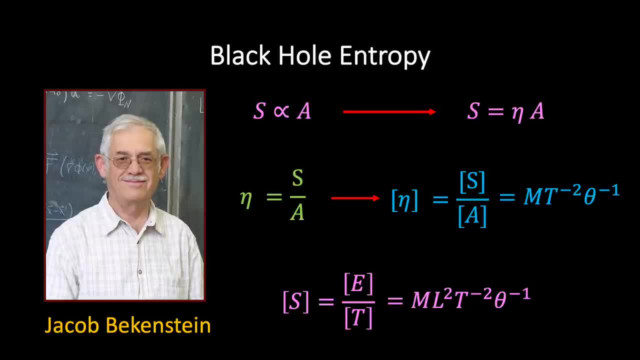 the fundamental constants we encountered earlier. But which constants shall we use in our dimensional analysis? Well, this is where we need to make an educated guess. Firstly, we are dealing with gravity in black holes, and so we should expect the gravitational constant and speed. 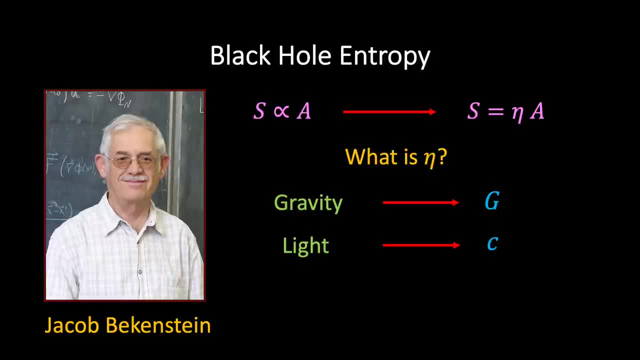 of light to be involved. Furthermore, since we are trying to construct an equation for entropy- and entropy is connected to thermodynamics, it makes sense to include Boltzmann's constant And finally, following the suggestion of Bekenstein in his original 1972 paper, we should also include Planck's. 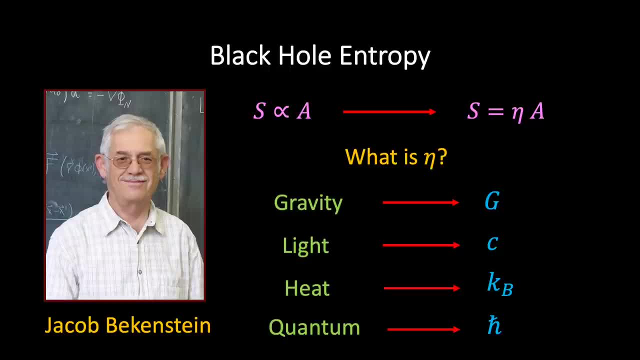 constant. As Bekenstein himself commented, we need not be alarmed at the appearance of H-bar in the expression for black hole entropy. It is well known that H-bar also appears in the equations for entropy of many thermodynamic systems that are conventionally regarded as. 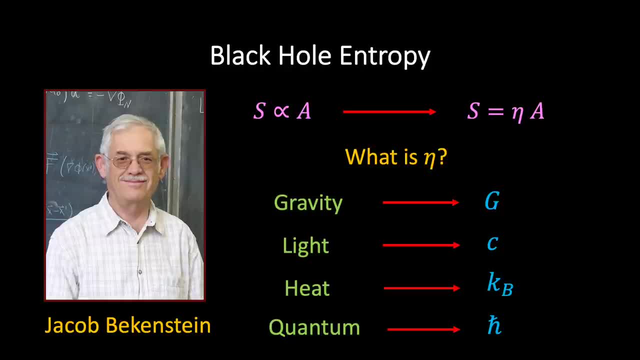 classical, for example the Boltzmann ideal gas. This is a reflection of the fact that entropy is, in a sense, a count of states of the system, and the underlying states of any system are always quantum in nature, And so, following in the footsteps of Bekenstein. 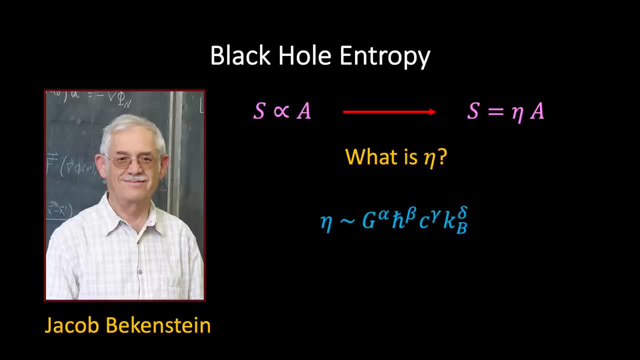 we will propose that eta can be written as g to the alpha, h-bar to the beta, c to the gamma times, k to the delta. So how do we determine alpha, beta, gamma and delta? Well, as we have already seen, 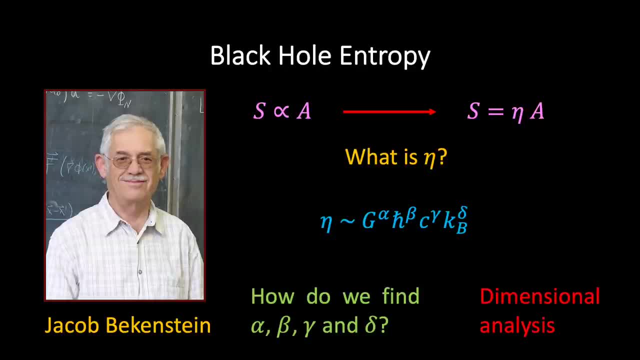 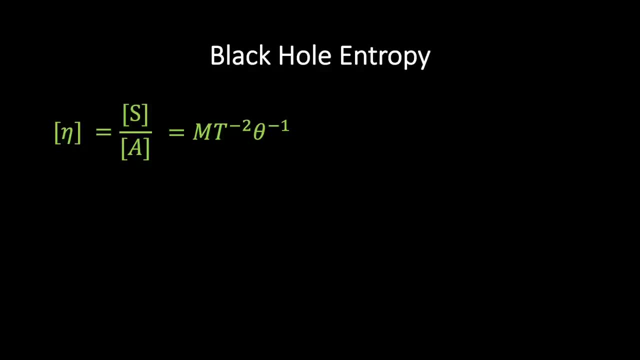 we simply need to apply the rules of dimensional analysis. So let's do that. Firstly, we have already calculated the dimensions of eta from the definition of thermodynamic entropy. Secondly, we know that the combined dimensions of g, h-bar, c and k must match. 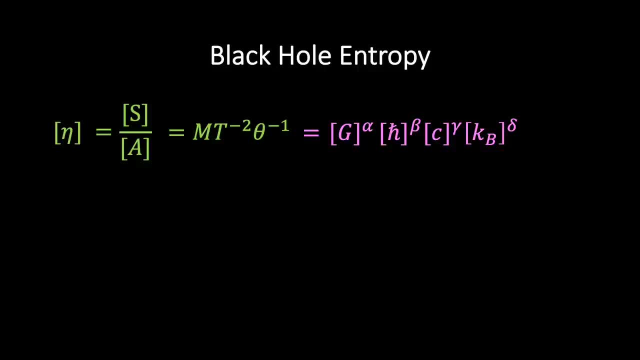 these. If we substitute the dimensions we calculated earlier for the fundamental constants, then we find the following yellow expression: If we then use the law of exponents to gather appropriate terms together, we can write this expression in the following form: Just like before, we can then match exponents on either side of the equation to form a set of simultaneous. 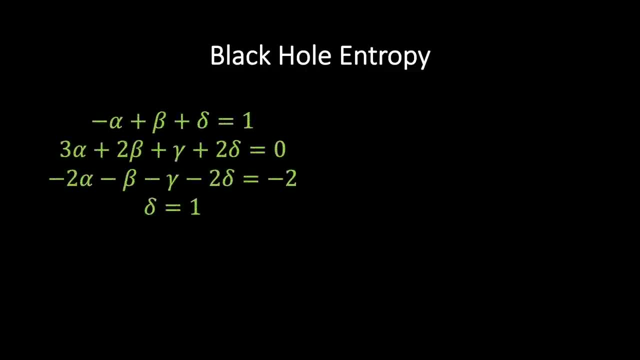 equations. If we do this, then we find the following set of constraints: We can then solve this set of simultaneous equations by substitution, and we find that alpha and beta equal minus one. If we then substitute these expressions back into the original equation proposed by Bekenstein, 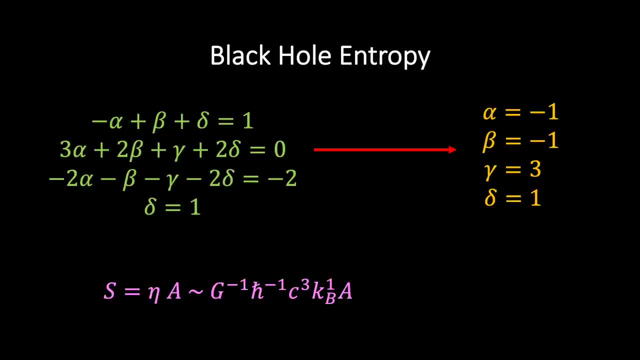 we find that, up to an undetermined numerical factor, the entropy of a black hole is proportional to the following expression: In 1974, using a subtle and sophisticated combination of general relativity and quantum field theory, Stephen Hawking was able to show that the exact form of the entropy equation 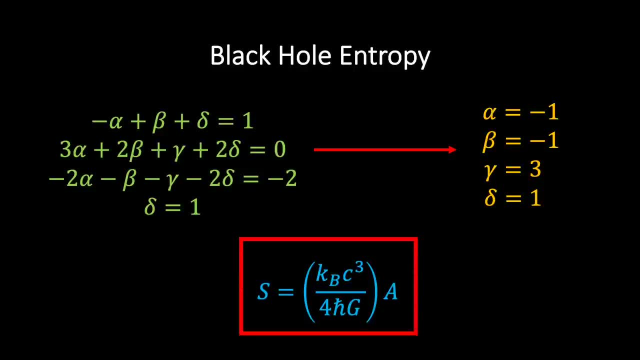 includes a numerical factor of exactly one, So we can then substitute these expressions back into the original equation proposed by Bekenstein. The expression for black hole entropy is written as: S equals k c cubed over 4. h bar g times the area of the event horizon, One of the most immediately striking aspects of this. 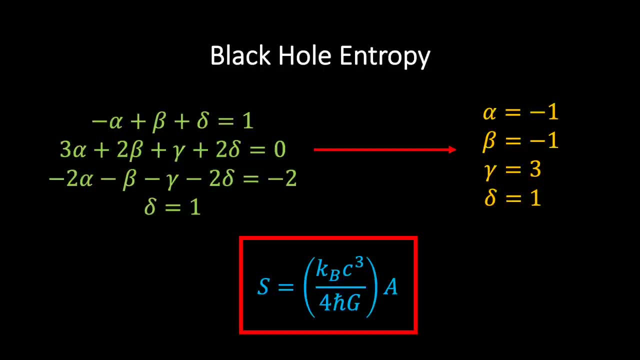 expression is that the entropy of a black hole is going to be incredibly large, since the equation contains a factor of c cubed in the numerator and both Planck's constant and Newton's gravitational constant in the denominator. So what is causing this large entropy value? 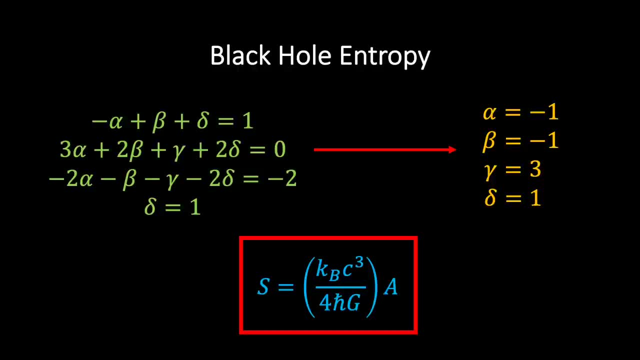 Well, according to Boltzmann, the entropy of a system relates to the number of possible microstates of the system. So if we apply this to black holes, it suggests that black holes should have some kind of microstructure which we can use to count states. 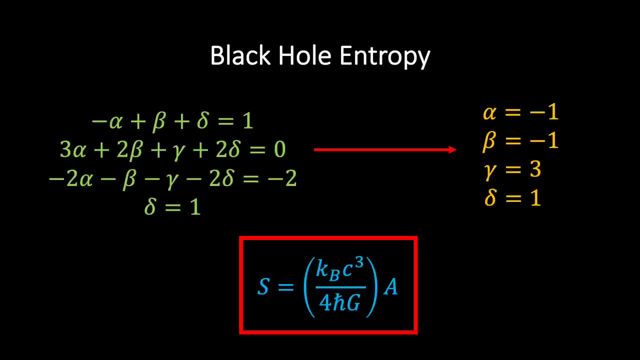 Furthermore, the presence of both Newton's gravitational constant and Planck's constant in the entropy equation suggests that these black hole microstates might have some type of value. This is something to do with the quantum theory of gravity. We will return to these interesting observations towards the end of this video, but for now, 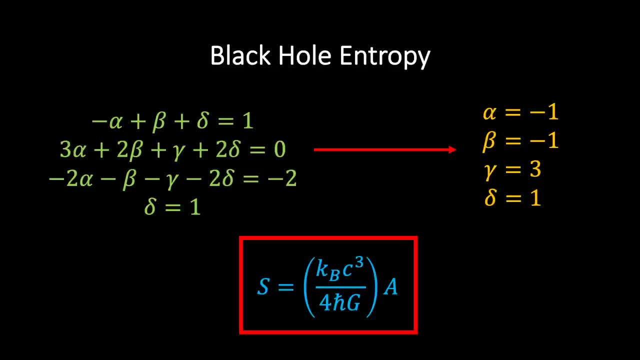 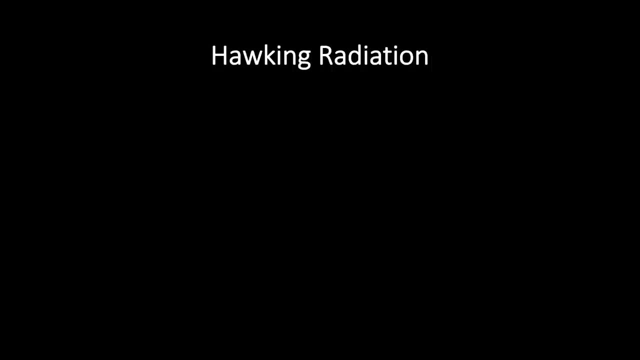 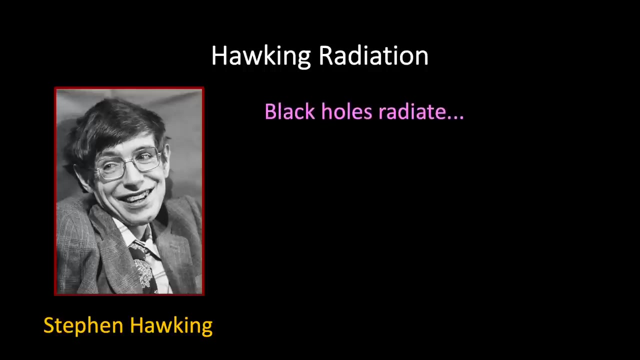 we wish to use the entropy equation to understand one of the most exciting predictions of 20th century physics: Hawking radiation. In 1974, Stephen Hawking discovered a remarkable fact about the universe: Black holes glow, emitting faint radiation, causing them to eventually evaporate and disappear. 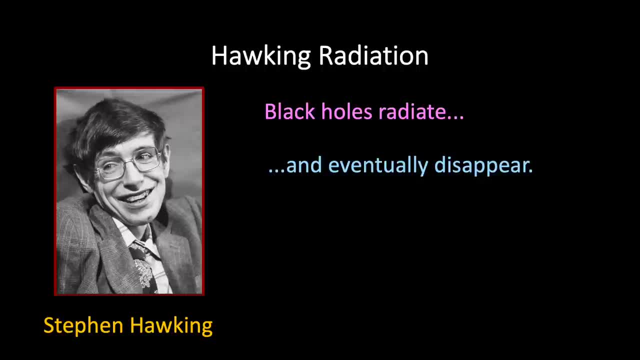 The example is this: The exact mechanism behind Hawking radiation involves a complex and subtle interplay between the curvature of spacetime caused by the event horizon and quantum fluctuations of the vacuum of empty space, a topic which I hope to return to in a future video. 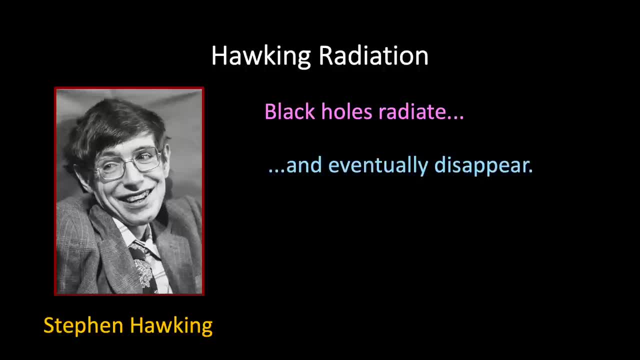 Hawking discovered that, since radiation appears to be emitted from the region of space surrounding the event horizon of the black hole, it should be possible to assign an absolute temperature to the black hole, the aptly named Hawking temperature. Furthermore, because mass and energy are seen as a constant, the black hole is not a black hole. 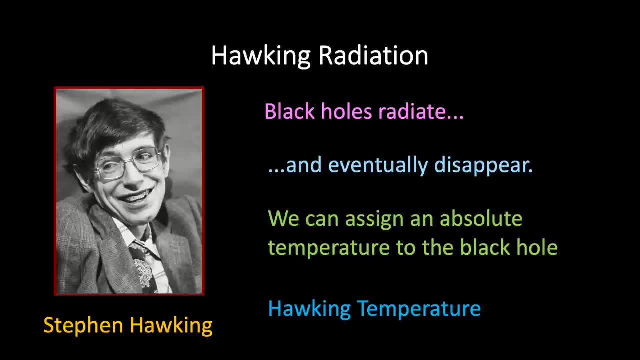 When a black hole radiates energy, it effectively loses mass and therefore should eventually evaporate. So let's now turn our attention to these remarkable discoveries and see if we can calculate the Hawking temperature and evaporation time of a black hole using our rudimentary toolkit. 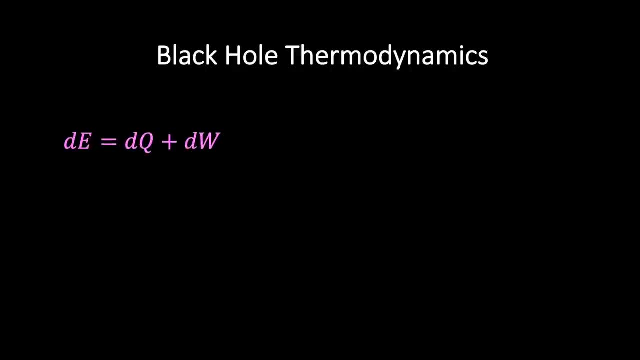 Our start point is to combine the first law of thermodynamics with the definition of thermodynamic entropy that we encountered earlier. Assuming that the black hole does no work on its surroundings, we can set w. w equals 0, and so we can write: dE equals T times dS, where dE refers to the change in energy of the black hole, T. 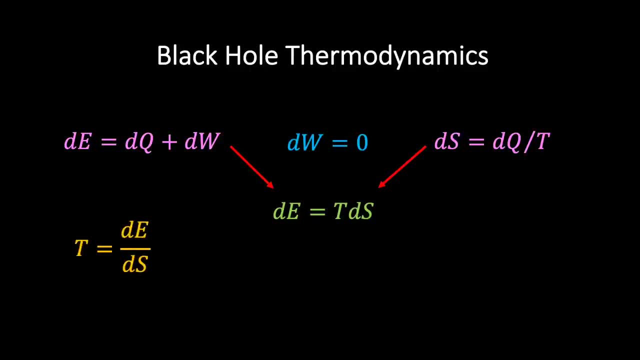 the thermodynamic temperature and dS the entropy. If we then rewrite this expression in terms of the temperature, we have that T equals dE by dS. Next, if we assume that the total energy content of the black hole is due to the incorporation of the black hole into the thermodynamic temperature, then the music of the black hole depends on whether intensity is maintained by the temperature right in this zone of the black hole. 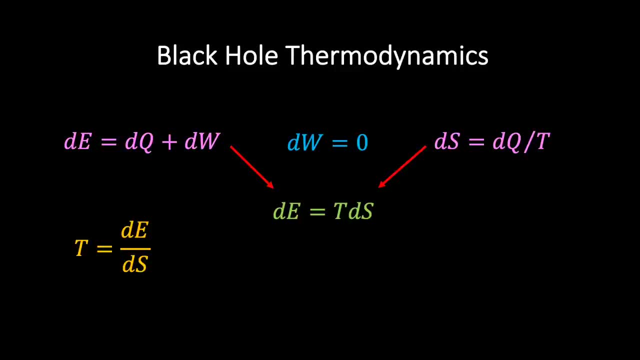 influences the black hole. Validating Transavas: kilograms per��oungness, rho mod nr to the mass contained within it, then we can use Einstein's famous equation to write: E equals mc squared. If we then combine this with the expression for T, we see that the 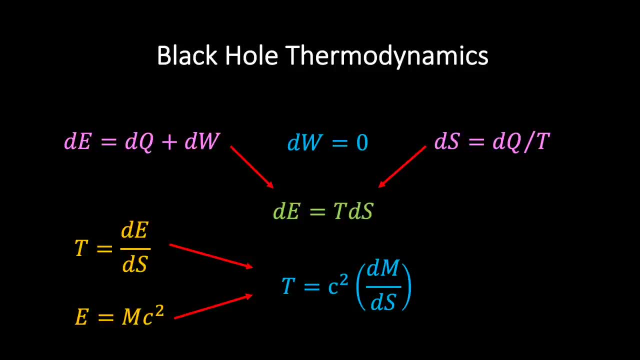 temperature of the black hole can be written in the following form, which we can then invert and write as c squared times the inverse of ds by dm. So we see that in order to calculate the temperature of our black hole, we need to differentiate the black hole entropy with: 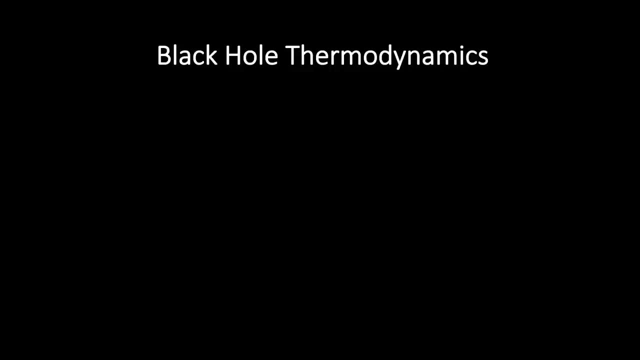 respect to mass, And so our next task is to rewrite the Bekingstein-Hawking entropy equation in terms of mass. To do that, we simply need to substitute the event horizon area equation into the entropy equation, and we find that S is proportional to the square of the black. 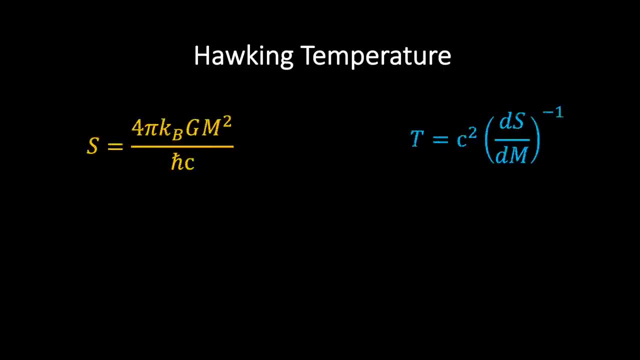 hole mass. If we then differentiate this entropy equation with respect to m, Try to find out how S is proportional to the square of the black hole mass, And so we'll. then we find the following green equation: and so we are now finally in a position to determine the. 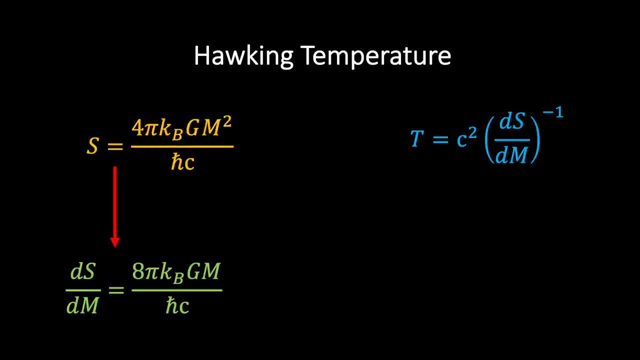 thermodynamic temperature of a black hole. We simply need to substitute this green expression into the equation we wrote for the thermodynamic temperature. If we do this, then we find that the temperature of our black hole can be written as h bar times c cubed divided by 8 pi kgm. 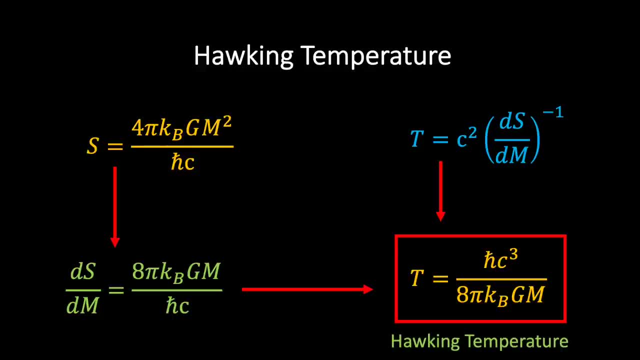 This temperature is known as the Hawking temperature of the black hole, and it's the temperature that we associate with the radiation being emitted from the black hole. One immediately striking feature of this expression is that the Hawking temperature is inversely proportional to the mass, and so the smaller the mass of a black hole, the higher the temperature, and therefore, 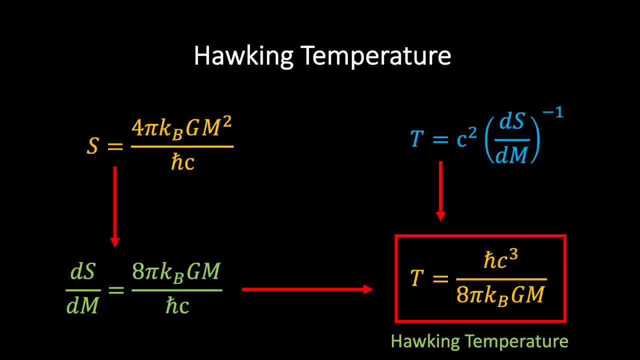 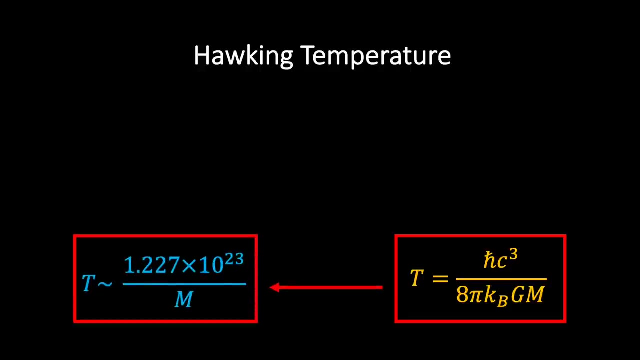 unlike most objects, a black hole's temperature increases as it radiates away its mass. But what kind of temperature is the Hawking temperature? What kind of temperatures are we talking about? If we sub in the values for the fundamental constants, then we find that the Hawking temperature can be approximated by the following blue expression: 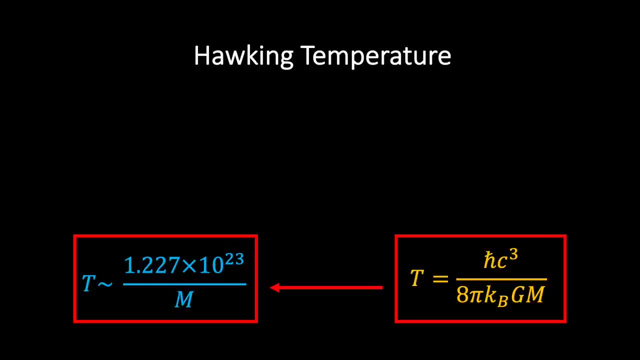 To get a sense of scale, the smallest stellar mass black hole that has so far been discovered has a mass of around three solar masses. If we insert this mass into the blue equation then we see that the Hawking temperature is around 2 times 10 to the minus 8 kelvin. 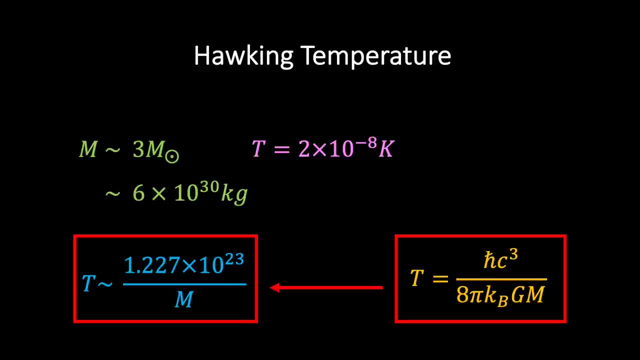 which is about 20 billionths of a degree. By way of comparison, we know that the temperature of the cosmic microwave background radiation is around 2.7 kelvin, and therefore a black hole of this mass would actually be absorbing far more energy than it emits and wouldn't begin to lose mass until the universe has. 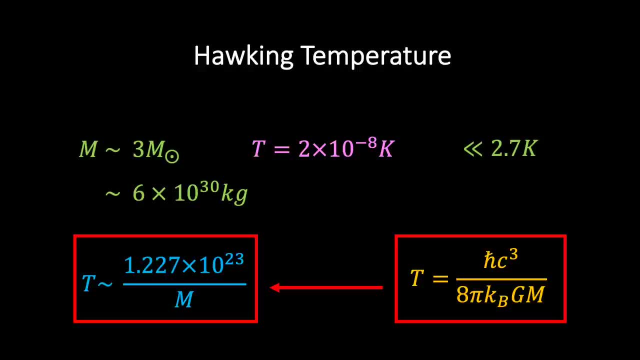 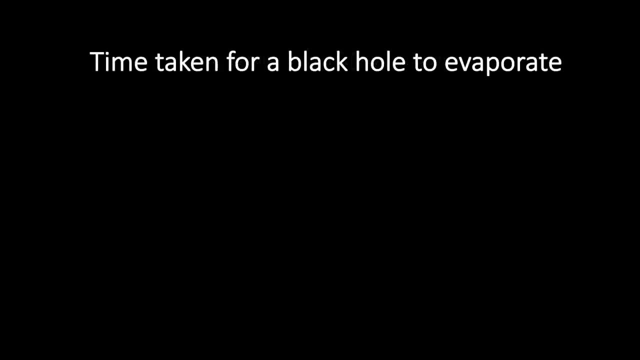 expanded sufficiently to reduce the temperature of the cosmic microwave background radiation. Okay, but let's for a moment assume that the universe has expanded sufficiently and the black hole begins to lose mass through Hawking radiation. How long will it take for all the energy of the black hole to radiate away? 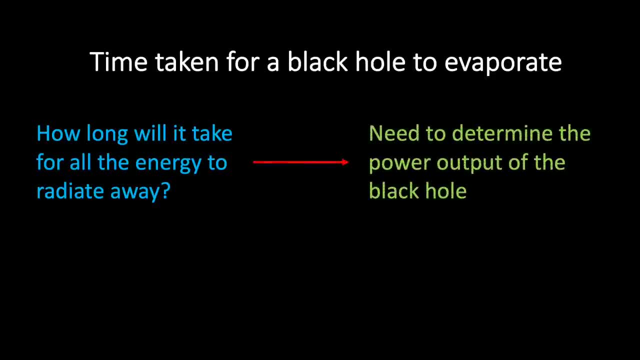 To answer this question, we need to determine the power output of the black hole, The rationale being that, since power is defined as energy per unit time, if we know the energy content of the black hole and the power output, then we can calculate the time taken for the energy to radiate away. 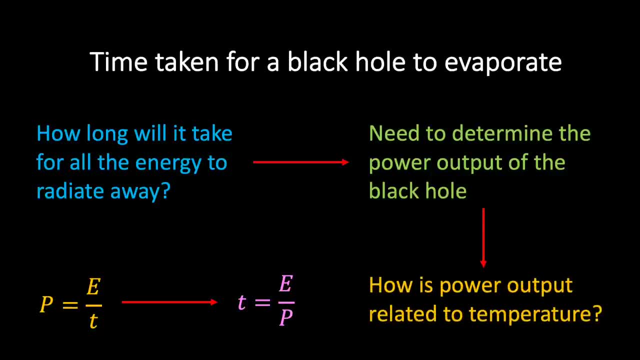 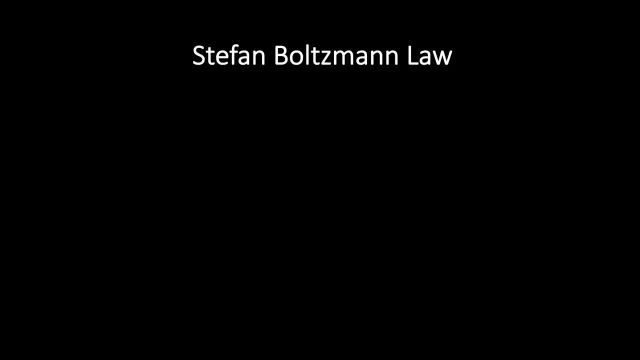 So our next task is to determine how the power output of a black hole relates to the Hawking temperature. To this we now turn. Our start point is to use dimensional analysis to estimate the power emitted per unit area from an object with temperature T. 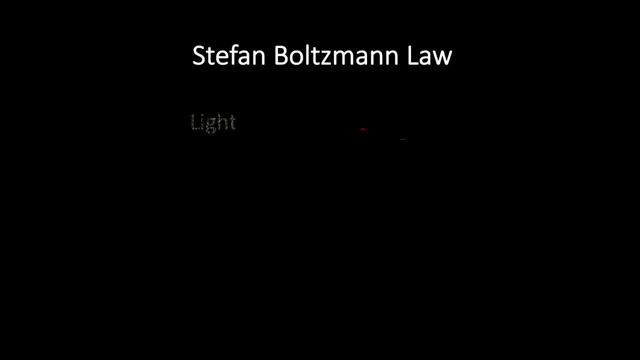 Since we're dealing with radiation, we should expect our equation to include the speed of light. and since we're dealing with heat, we expect our equation to include Boltzmann's constant along with the temperature T. And finally, we'll also include Planck's constant. 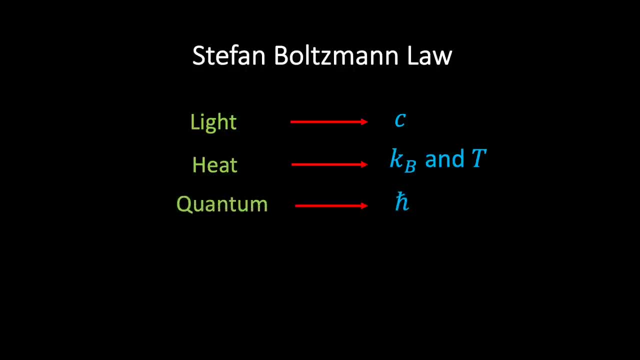 After all, it was by explaining the radiation properties of hot objects that Planck was first led to introduce the constant that bears his name. So let's begin by assuming that the power per unit area depends on the fundamental constants. in the following way: As before, we can determine the constants alpha, beta and gamma and delta by matching the dimensions on either side of the equation. 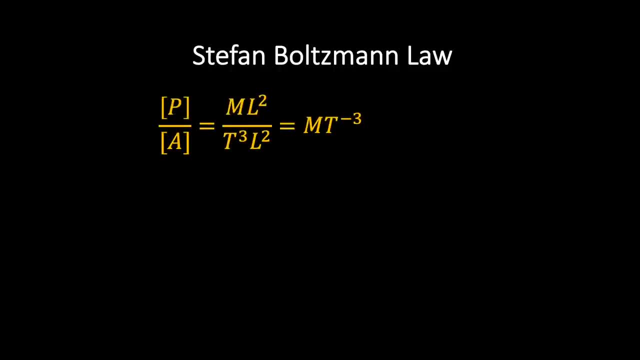 We see that the left-hand side has two constants. We see that alpha has the dimensions of M, T to the minus 3, whereas the right-hand side is given by the following blue expression: If we expand out the brackets and simplify, then we find the following green expression: 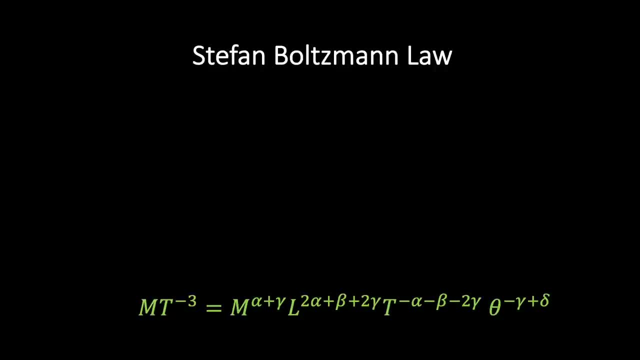 If we then match up the exponents on either side of the equation, we find the following set of simultaneous equations which can be solved to find that alpha equals minus 3, beta equals minus 2, and gamma and delta equal 4.. 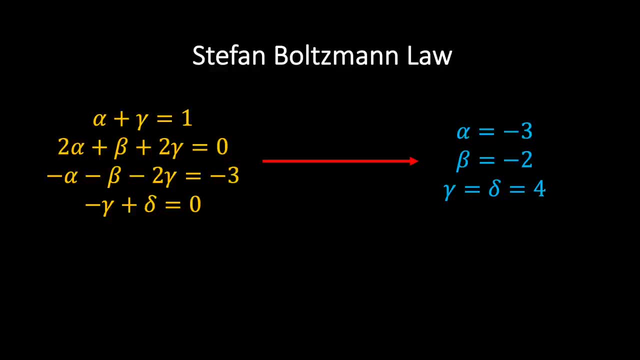 And therefore we see that the potential for the function of the black hole is the following: And therefore we see that the power per unit area is given by the following green equation, which you might recognize as the famous Stefan-Boltzmann relation: 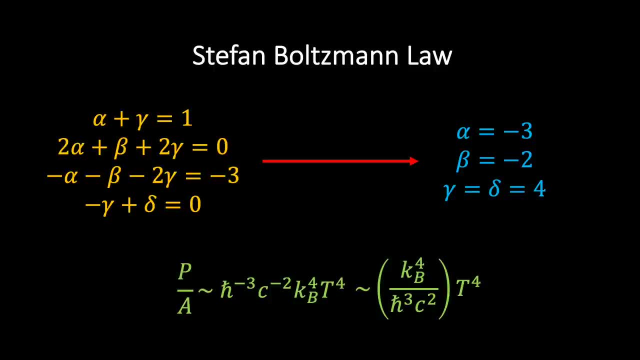 which says that the power per unit area of a hot object is proportional to the fourth power of the temperature. A detailed quantum mechanical calculation yields the well-known exact result, and we see that the numerical coefficient is equal to pi squared over 60.. If you're interested in how this result is derived, I refer you to my video on the cosmic microwave background radiation. 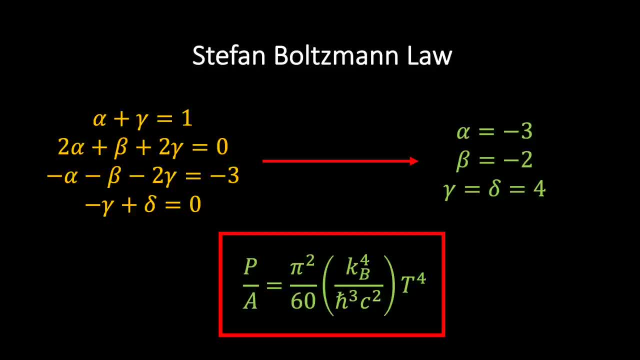 For our purposes, let's use the Stefan-Boltzmann relation to estimate the power output of our three solar mass black hole, which, if you recall, had a Hawking temperature of 2 times 10 to the minus 8 Kelvin. 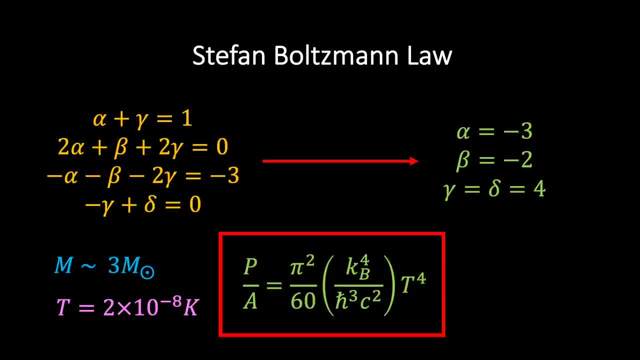 If we plug in the numbers, then we find that the power output of the black hole is incredibly small: around 10 to the power of minus 29 watts. For comparison, our Sun has a power output of around 10 to the power of 26 watts. 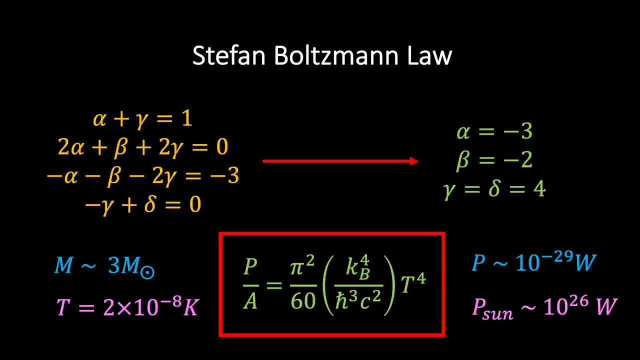 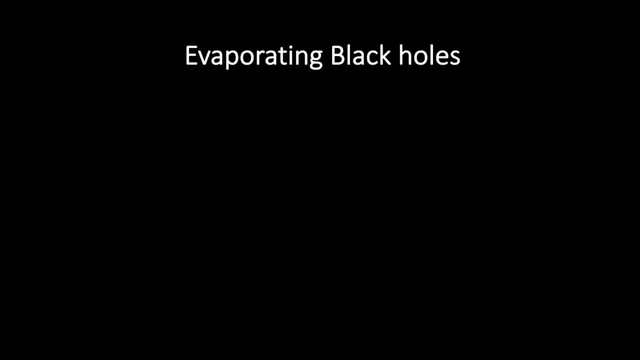 Given the incredibly small power output of a black hole, we might expect that it will take a very long time for a black hole to evaporate. But exactly how long? To answer this question? we first note that because the power of the black hole will be changing with time. 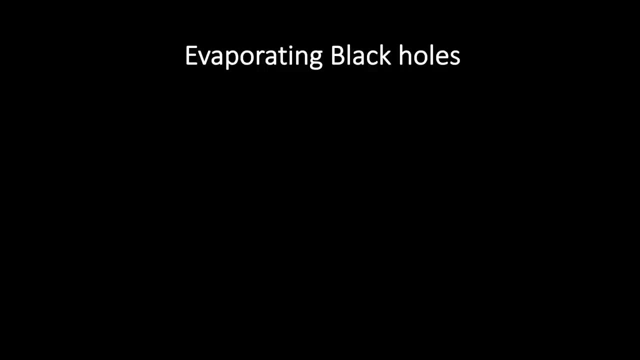 we will need to express the power relation in differential form as dE by dt. The appearance of the minus sign is due to the fact that the power of the Hawking radiation is the rate of energy loss of the black hole. Next, we need to take the Stefan-Boltzmann relation and rewrite this in terms of the mass of our black hole. 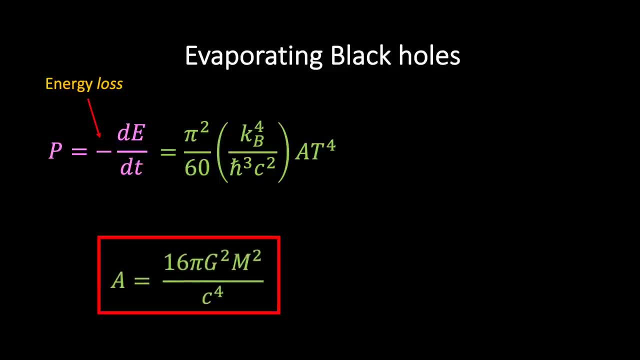 To do this, we need to substitute the expressions for the event horizon area and Hawking temperature that we've already met. If we do this, then we find the following blue equation: Note that as the mass of the black hole decreases, the power output. 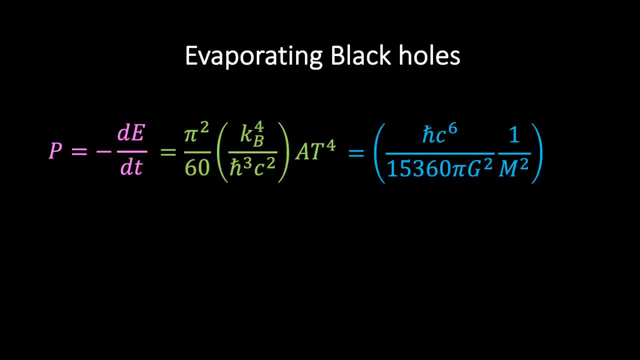 will actually increase. Next, we will rewrite the energy in terms of the mass by using Einstein's equation: E equals mc squared, where m is the total mass of the black hole. If we sub this into the differential expression, then we can write our power equation in terms of the rate of change of mass. 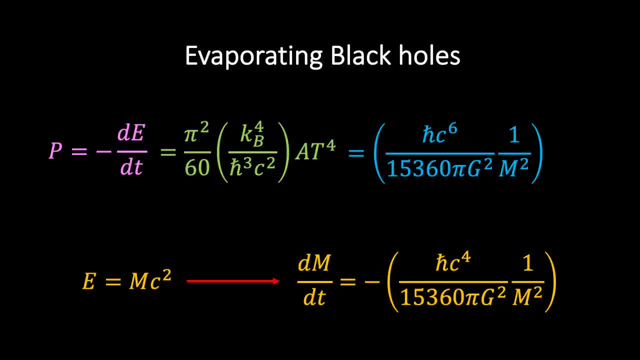 instead of the rate of change of energy. This makes sense because the right-hand side of the equation is expressed in terms of the mass. In order to solve this equation equation, we will use the method of separation of variables. The first step is to rearrange. 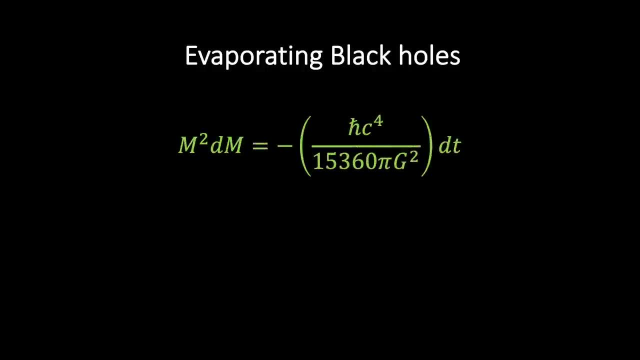 this equation so that we have m squared, dm on the left hand side and dt on the right hand side. If we then integrate both sides of this equation with respect to t, we find the following yellow expression: where t equals zero refers to when the black hole starts. 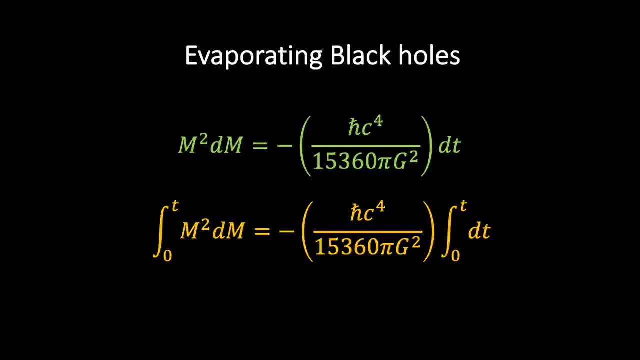 evaporating and t refers to some later time. Integrating m squared will give a factor of m cubed over three on the left hand side, whereas integrating with respect to time on the right hand side will give rise to a factor of t. If we then insert the limits, 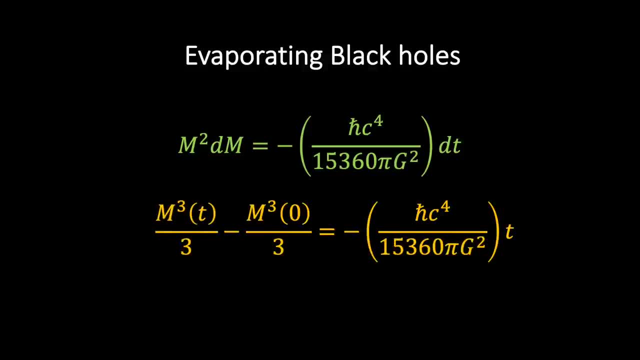 we find the following result: We can then use this expression to estimate the time taken for an isolated black hole to evaporate completely, In other words, the time taken for a black hole to lose all of its mass. To do this, let's define t equals t- evaporation as the moment. 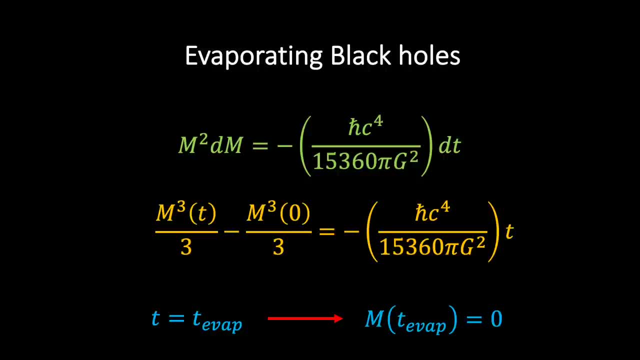 in time when the mass of the black hole has reduced to zero. If we then substitute this information back into our equation and simplify, we find the following green equation expressed in terms of the evaporation time. Finally, if we rearrange for t, then we find that the evaporation 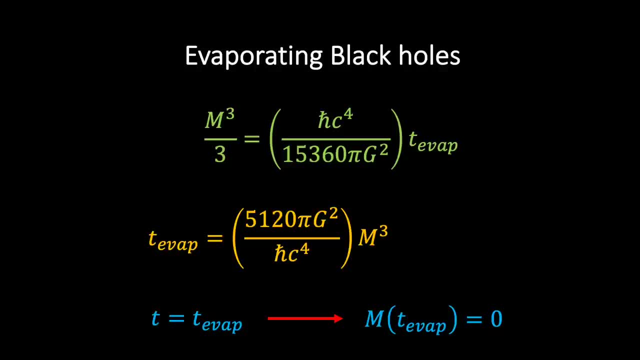 time is proportional to the cube of the mass of the black hole. Plugging in the values for the constants, we find that the evaporation time is roughly equal to 10, to the power of minus 16 times m cubed, where m is the mass of the black hole at the start of the evaporation. 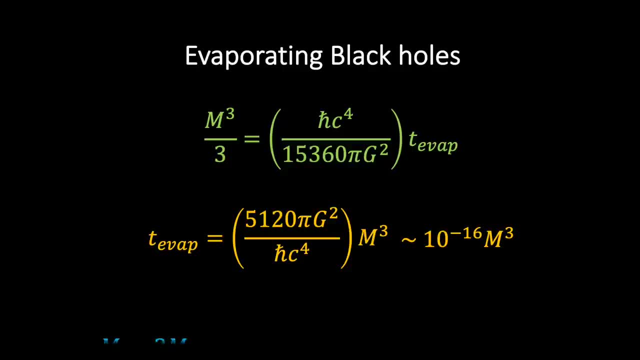 process. If we again consider a black hole of three solar masses, then we find that the evaporation time is of order 10 to the 68 years. Considering the universe is believed to be around 13.8 billion years old, we see that the time taken for evaporation is many. 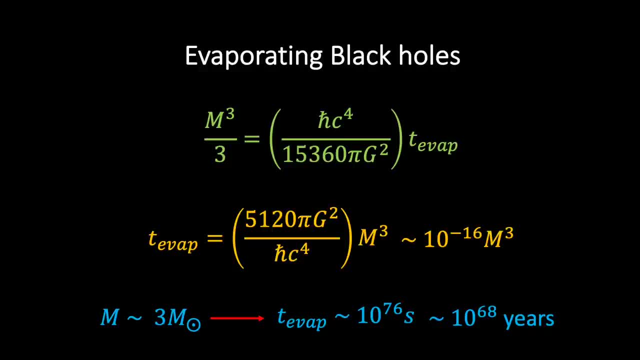 many orders of magnitude larger than the age of the universe, and therefore a solar mass black hole is likely to be around 13.8 billion years old, So we can then use this equation to calculate the time taken for an isolated black hole to lose all of its mass. To do this, 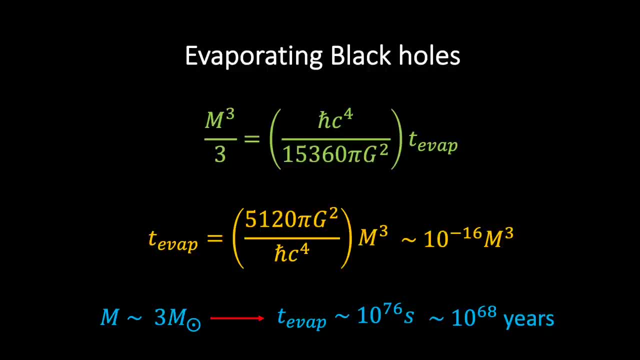 the universe will have to be around long after all the stars in the universe have died out, making it highly unlikely that we will ever observe the black hole's final farewell. So is there any way that a black hole might evaporate in a shorter period of time? Well, 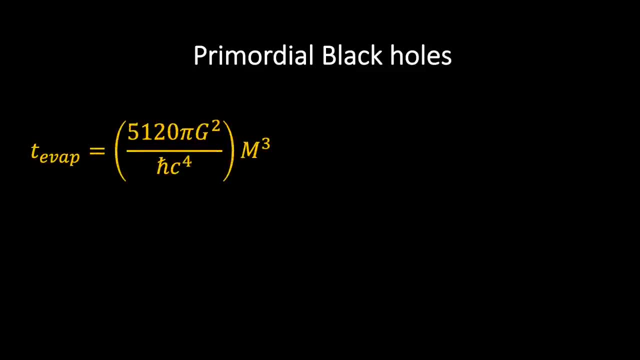 a quick glance at the black hole evaporation equation reveals that the only factor affecting the evaporation time is the black hole mass. Could it be possible, then, that a black hole with sufficiently small mass, perhaps created in the early universe, has an evaporation? 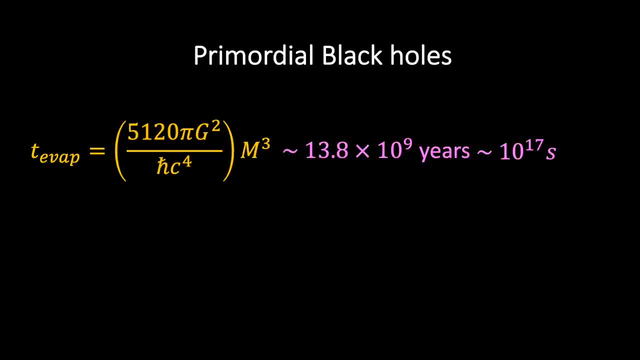 time roughly equal to the age of the universe. That way, the primordial black hole could be coming towards the end of its life at the present moment, and we might be able to detect the dying radiation burst of the black hole. Well, it turns out that it's relatively straightforward to estimate what the 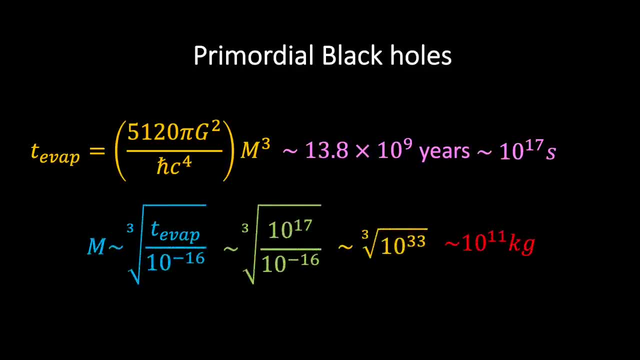 mass of such a black hole would need to be. We simply rearrange the black hole evaporation equation for M and substitute the age of the universe, and we find that the initial mass of the black hole must have been around 10 to the power 11 kilograms, which is roughly equivalent to the mass of an asteroid. 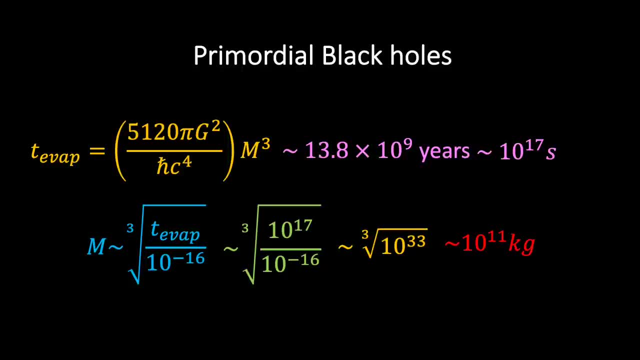 Now, according to our current laws of physics, a black hole of such small mass could not have formed as a result of stellar death, as is typical for black hole formation. Rather, it's conceivable that such primordial black holes might have formed by random fluctuations in the very early universe, and if so, these: 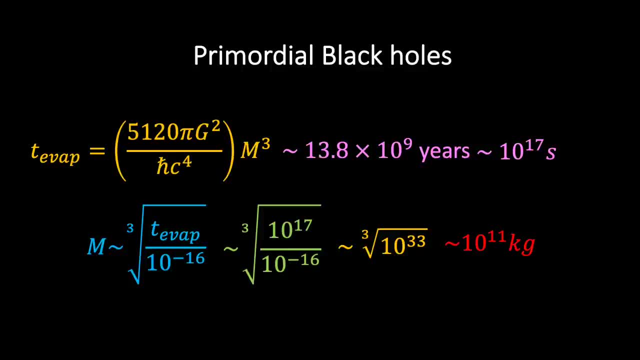 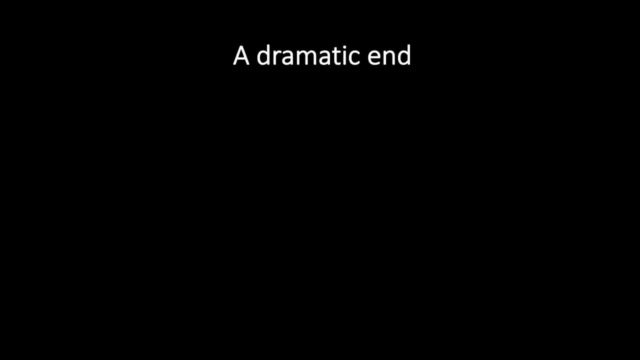 primordial black holes should be coming towards the end of their lives. So what exactly happens during the last few moments of a black hole's life? Well, we can estimate the amount of energy released in the last second of a black hole's life, because this is equal to the energy. 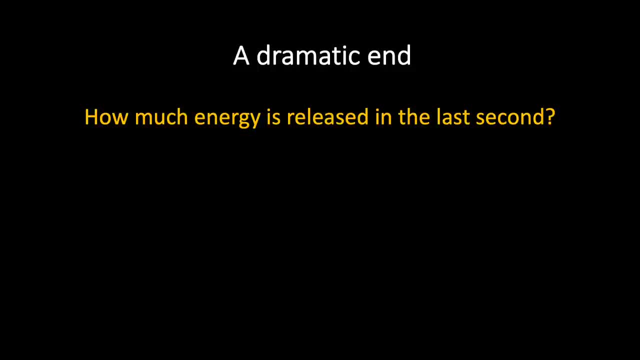 equivalent of the mass of a black hole whose lifetime equals one second. So if we sub in t equals 1 into the evaporation equation, we find that the black hole radiates the energy equivalent of 10 to the power 5 kilograms of mass during its final second. We can work out how much energy. 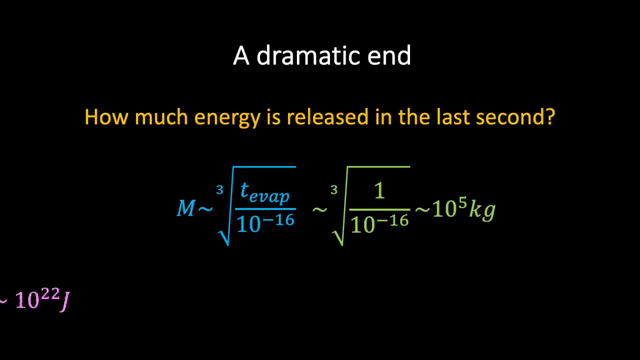 this corresponds to, using Einstein's famous equation, equals mc- squared, and we find a value of around 10 to the power of 22 joules. By way of comparison, the largest nuclear weapon ever detonated on earth, known as the Tsar bomber, released 10 to the 17 joules of energy, and so we see that the energy released in 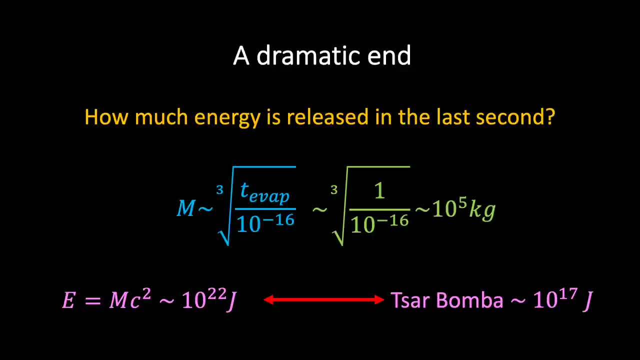 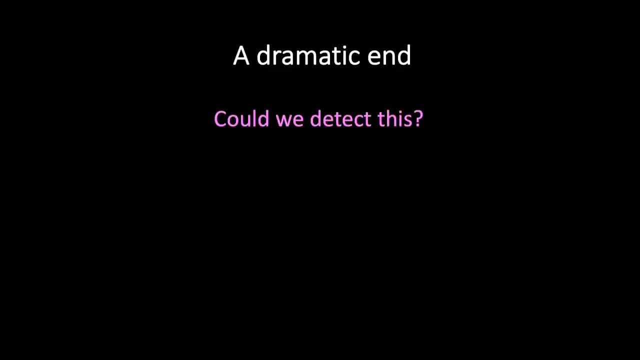 the final one second of a black hole is roughly equivalent to the energy released by 100,000 Tsar nuclear bombs. So could we detect this? The release of this much energy in one second might just be observable here on earth, Although it's only a fraction of a percent of the luminosity of. 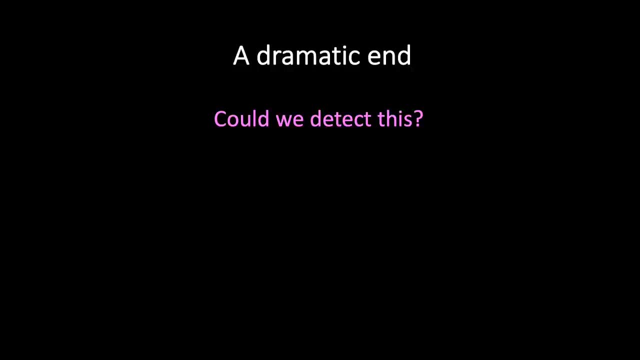 the sun, it would come out in a characteristic burst of gamma rays which could hopefully be detected. But how do we know it would be gamma rays? Well, that comes from the Wien displacement law, which says that for an object at temperature t, the wavelength corresponding to peak intensity 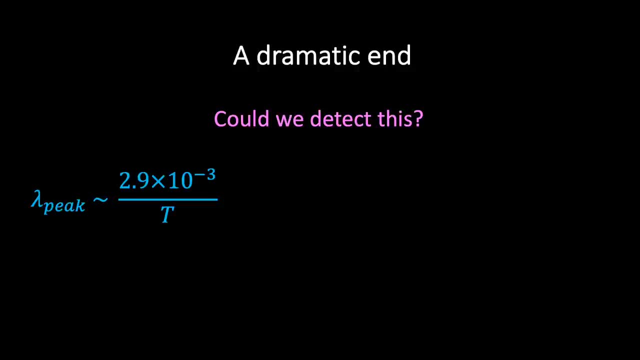 emission is inversely proportional to the temperature t. I refer you to my video on the cosmic microwave background radiation for a derivation of this result. For our purposes, we can estimate the wavelength of peak emission by inserting the Hawking temperature corresponding to a black hole of mass 10 to the 5 kilograms, and we find that the 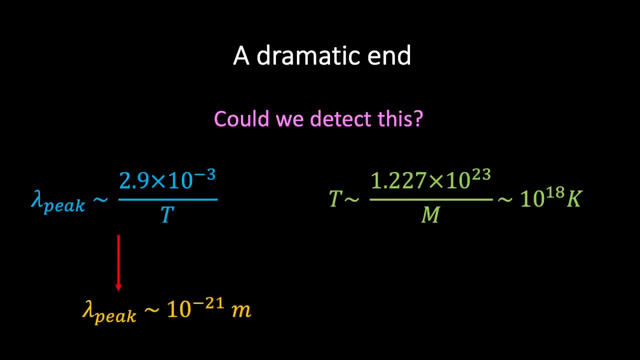 peak wavelength is of order 10 to the minus 21 meters, which is in the high energy gamma wavelength range of electromagnetic radiation, and therefore the hope is that it should be possible to detect this characteristic burst of gamma radiation which signals the last few moments of an evaporating black. 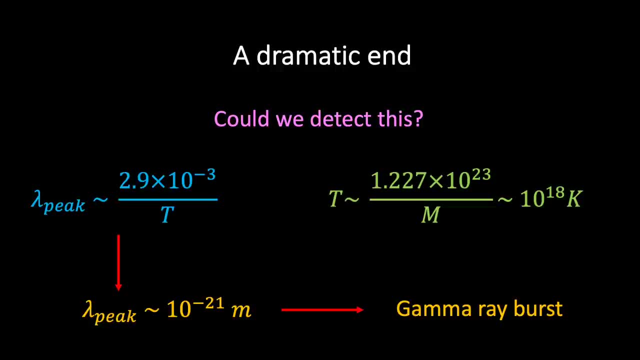 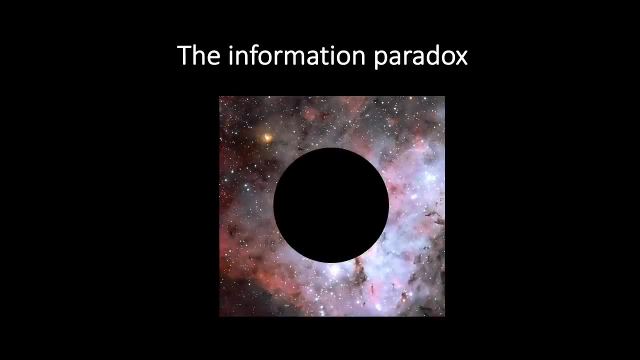 hole's life. It's worth noting that so far, nothing of this nature has ever been observed and therefore, at this stage, primordial black holes represent a purely theoretical idea. I would like to end by briefly discussing another important theoretical consequence of Hawking radiation, the famous black 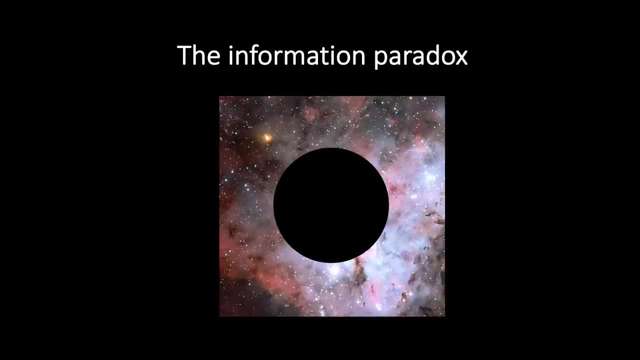 hole information paradox. Soon after Hawking's theory of black hole radiation. Hawking's theory of black hole radiation, he recognized a serious problem. Imagine throwing a laptop or a book or even a human being into a black hole. What happens to all of this information? The problem that 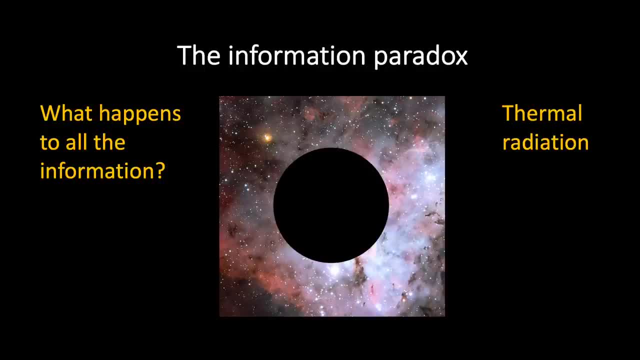 Hawking recognized is that the thermal radiation emitted from a black hole as it evaporates has no memory whatsoever of what went into the black hole in the first place. As we've already seen, only the mass, and therefore temperature, of the black hole determines what type of radiation is emitted, and this would seem to imply that information has been. 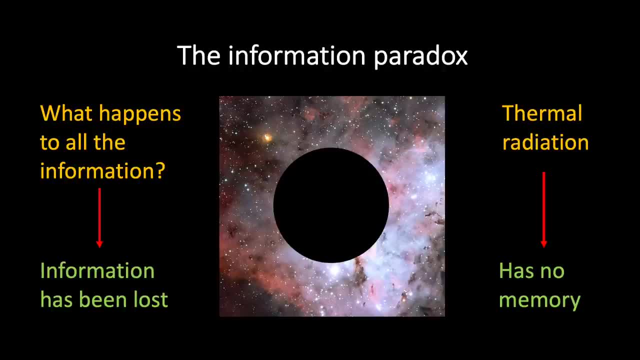 lost. In other words, we cannot use the Hawking radiation emitted from a black hole to reconstruct the information content of what originally fell inside. Now, this might not immediately strike you as a problem. however, the irretrievable loss of information conflicts with one of the basic 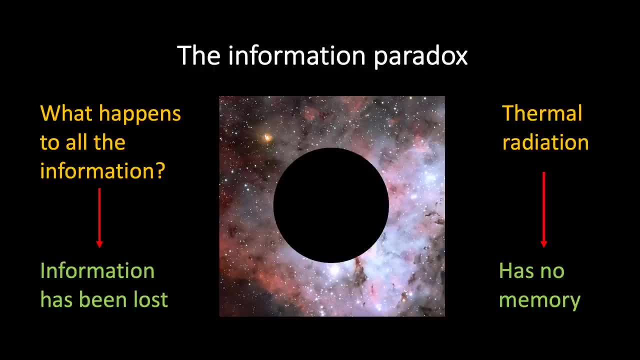 postulates of quantum mechanics. According to the Schrodinger equation, physical systems that change over time cannot create or destroy information, a property known as unitarity. This apparent contradiction between general relativity and quantum mechanics is the information paradox. So either quantum mechanics is wrong or the information somehow gets out of. 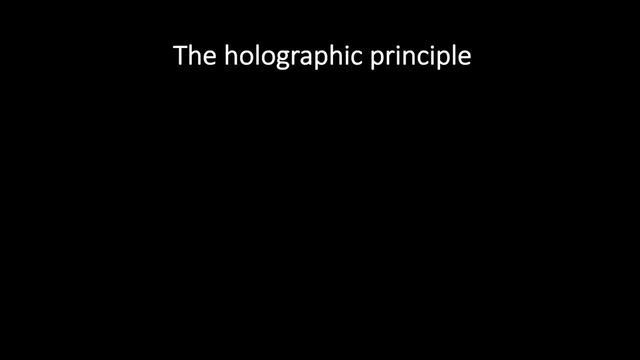 the black hole. One possible solution to the problem is known as the holographic principle, which suggests that the information content of a black hole is somehow encoded on the event horizon of the black hole. So let's look at this suggestion in a bit more detailMarcin. 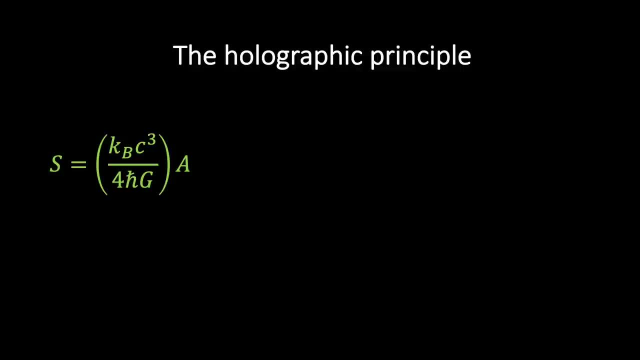 fichardde. So what could these fundamental microstates be? To shed some light on this, notice that we can rewrite the Marcinfichardde- Mrs Hall viens- entropy equation in terms of the Planck length which, if you recall, is believed to be the 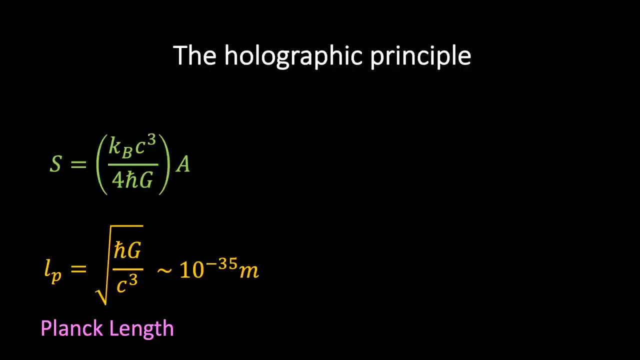 smallest meaningful distance that we can probe in nature. If we square the Planck length, we get the Planck area and notice that the Planck area is actually contained within the Bekenstein-Hawking relation. In particular, we can write the entropy as s equals k over 4 times the area of the horizon. 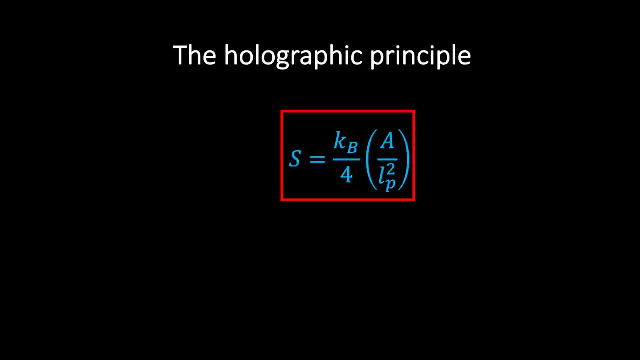 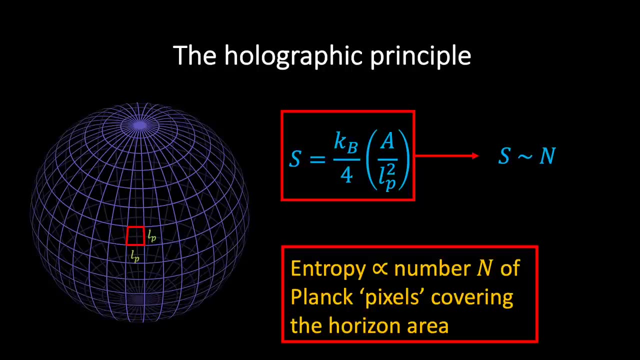 divided by the Planck area. So we see that the entropy of a black hole is proportional to the number of Planck areas that would cover the area of the black hole event horizon. So what does this mean? Well, perhaps we could use these Planck-sized pixels to somehow encode the information that has 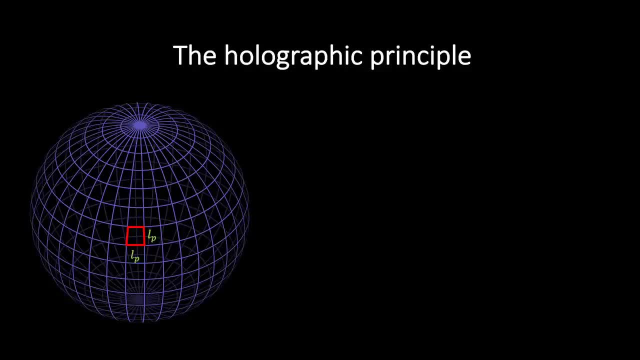 fallen into the black hole. More specifically, imagine that each Planck-sized cell corresponds to one bit of stored information. So, for example, if we were to use a Planck-sized cell, we could encode two possible states corresponding to 0 and 1.. With two bits or two cells, we can describe: 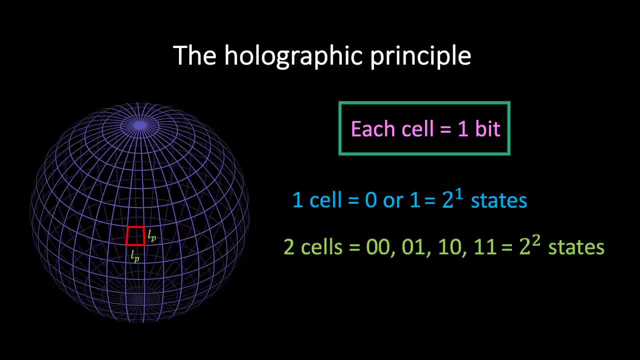 four states corresponding to 00,, 01,, 10, and 11.. Continuing this pattern, we see that with n bits or n cells, we can describe 2 to the n states corresponding to the 2 to the n sequences of: 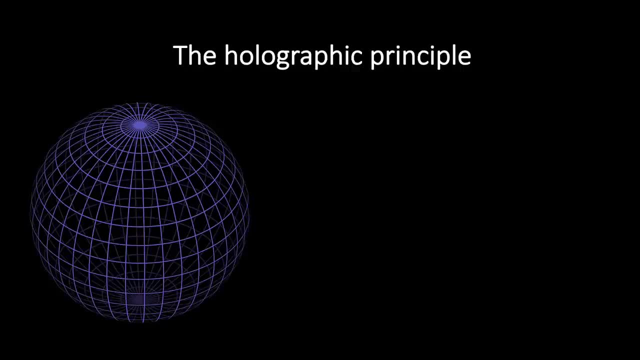 binary digits, Then, according to this pattern, we can encode two possible states corresponding to Boltzmann. the entropy of the system would be equal to Boltzmann's constant multiplied by the logarithm of the number of microstates corresponding to a particular macrostate. Well, if we take 2 to 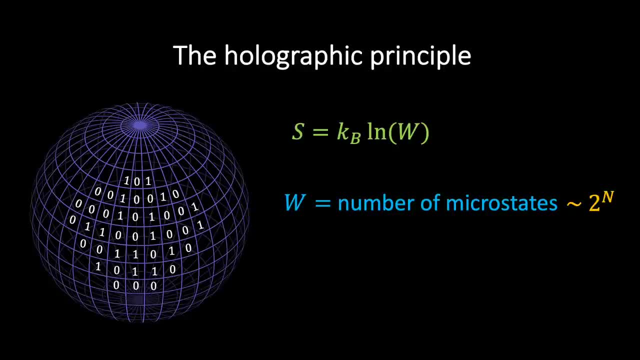 the n as the number of microstates, then we see that the entropy would be proportional to the logarithm of 2 to the n. We can then use the logarithm rule for exponents to show that the log of 2 to the n is proportional to n, And we have already established that the number of cells 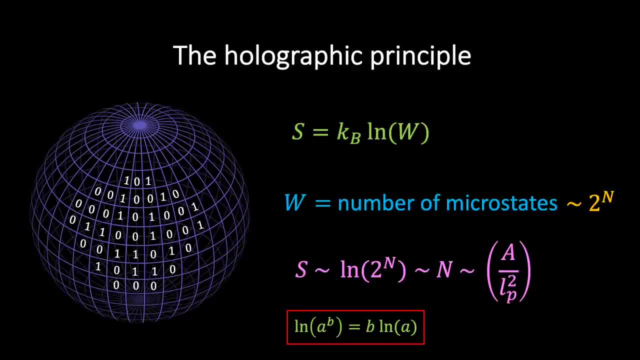 is proportional to the area of the black hole event horizon. and so we see, we recover the Bekenstein-Hawking relation To get a sense of just how much information a black hole could store using these Planck-sized cells. let's, for the purposes of illustration, imagine that we have 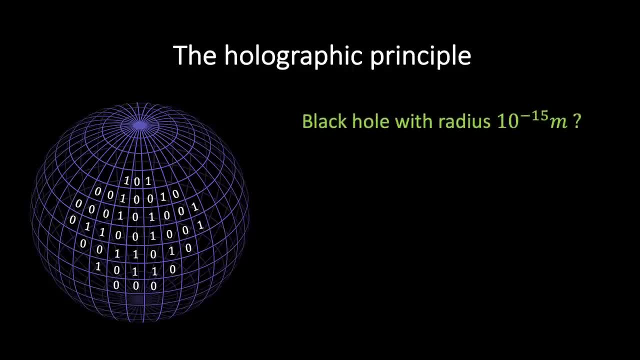 a tiny black hole the size of a proton, with a radius of order 10 to the minus 15 meters. We can then estimate the number of bits as the ratio of the area of the event horizon to the Planck area, and we see that we can. 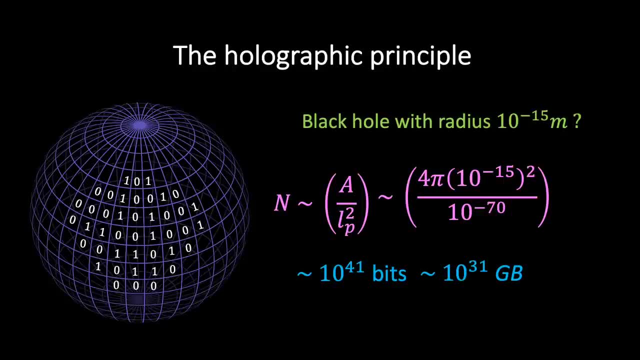 for the purposes of illustration, estimate the number of bits as the ratio of the area of the event horizon to the area of the event horizon, which is roughly 10 to the power 41 bits, which is roughly 10 to the 31 gigabytes. Compare this to the total data storage on all the computers in the world. 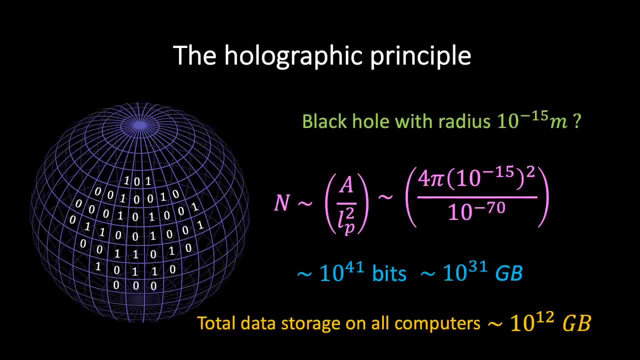 which is of order 10 to the 12 gigabytes, and we see that a proton-sized black hole could contain more information than all the world's computers by an unimaginably large factor. This general idea that information is stored on the black hole horizon is known as the holographic principle. 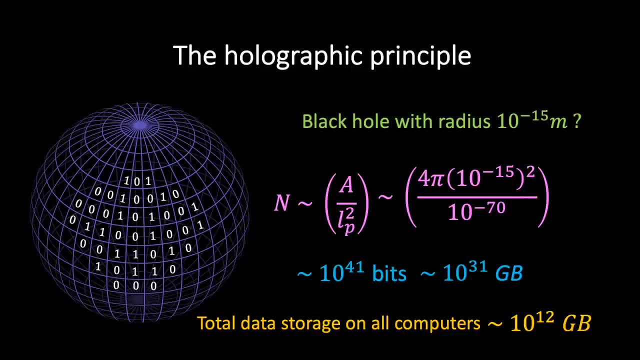 and that information that falls into a black hole is somehow encoded on the two-dimensional boundary like a hologram, And therefore, according to this set of ideas, the information swallowed by a black hole could be completely restored during the process of quantum evaporation, since it always 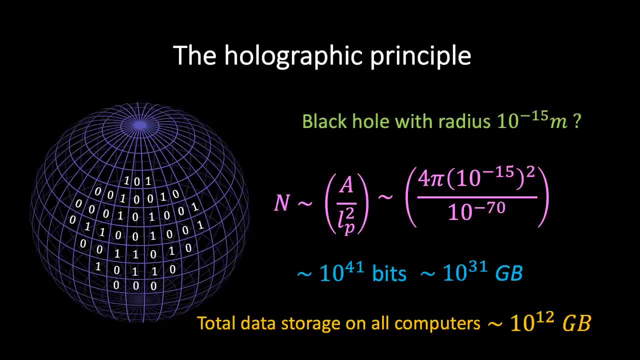 existed on the boundary of the black holeThe exact mechanism explaining how this restoration of information takes place is still an open question in theoretical physics, but there has been significant progress over the past 30 years to come. Thank you for watching and please give us a like and subscribe and hit the bell button if you liked the video. Thank you for watching. 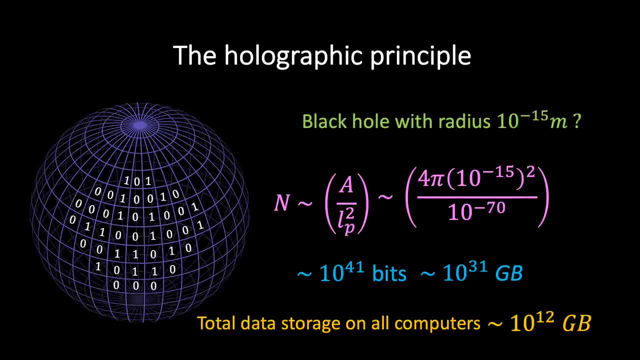 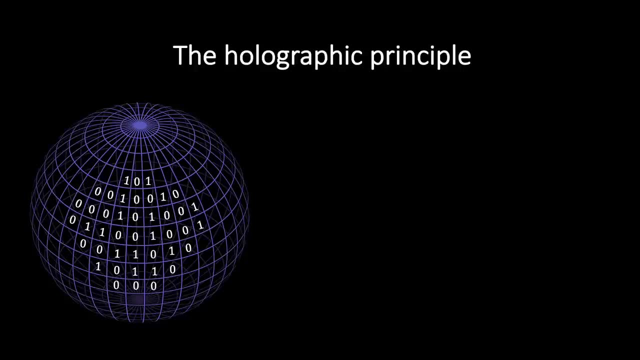 years to flesh out and generalize the holographic principle, especially within the context of string theory. The remarkable conclusion that comes out of this line of reasoning is the realization that, in order to describe what is going on in a volume of space, we need only concern ourselves with the 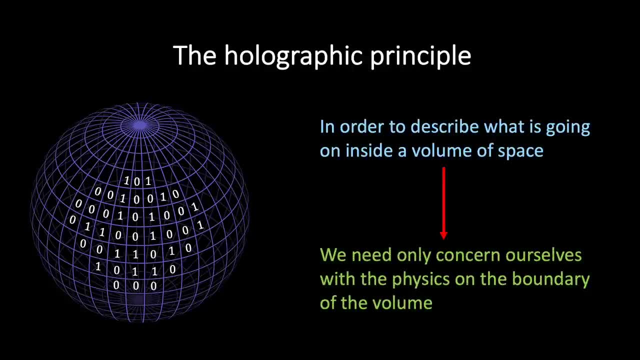 physics that resides on the boundary of the volume. You can think of a region of space as being surrounded by tiny plank-sized pixelated cells, and when things move around inside the volume, that information is somehow encoded in those cells. You can picture them lighting up As you. 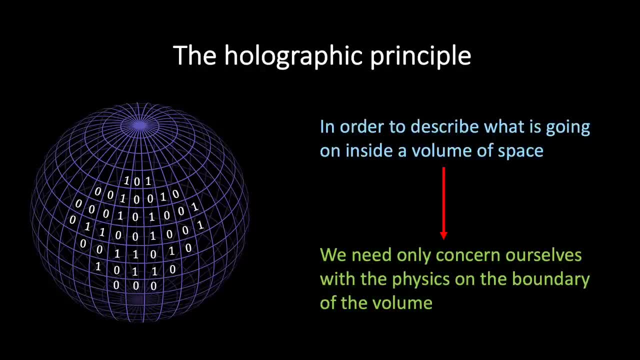 put more stuff inside the volume of space, more of the pixels light up and at the exact moment, just before the volume of space collapses to form a black hole, all of the pixels have lit up. In other words, all of the information is at the boundary, not inside the space. What controls? 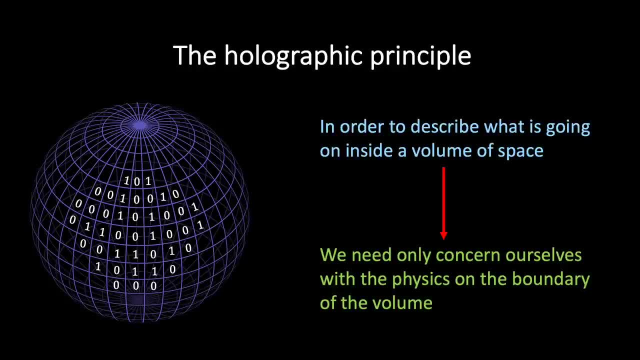 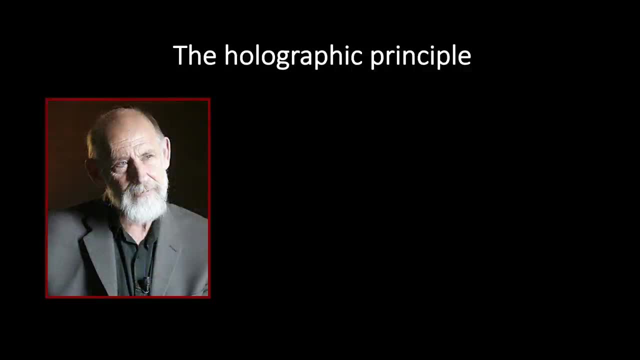 the physics lives on the boundary of the space, and this is the essence of the holographic principle. A detailed discussion of the holographic principle within the context of string theory will no doubt form the basis of a future video, But for now, I would like to leave you with the words of one of 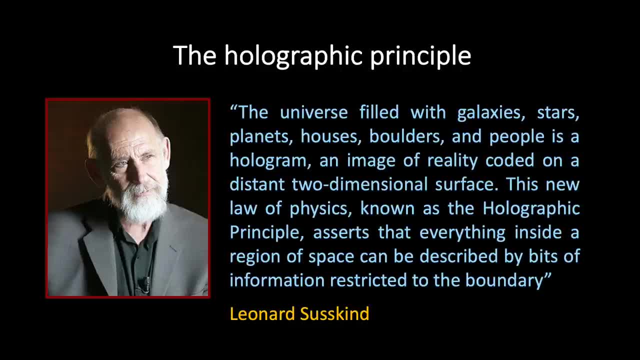 the founding fathers of the holographic principle, Leonard Susskind. The universe filled with galaxies, stars, planets, houses, boulders and people is a hologram, an image of reality coded on a distant two-dimensional surface. This new law of physics known as the holographic principle,